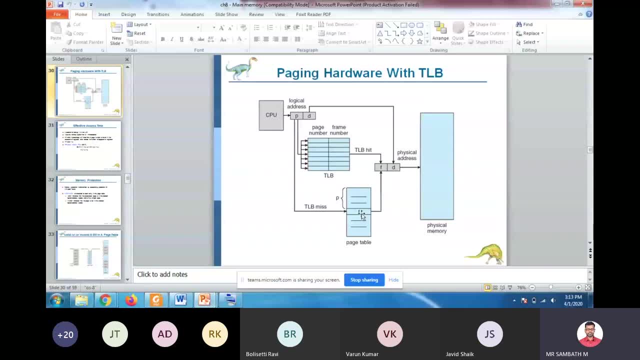 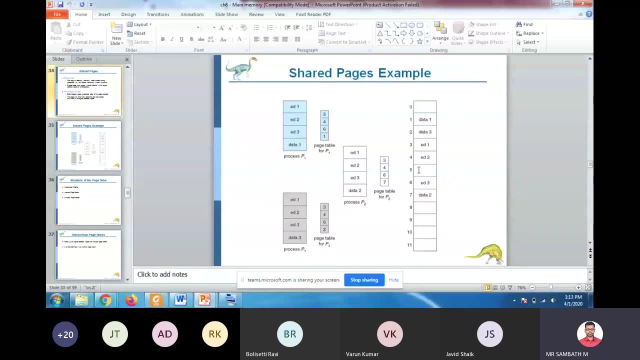 Then it will combine this and then it will generate the physical address. Then we have something called page tables, The types of page tables we have. The first one is hierarchical paging. The second one is hashed page table. The third one is inverted page tables. You will see one by one. 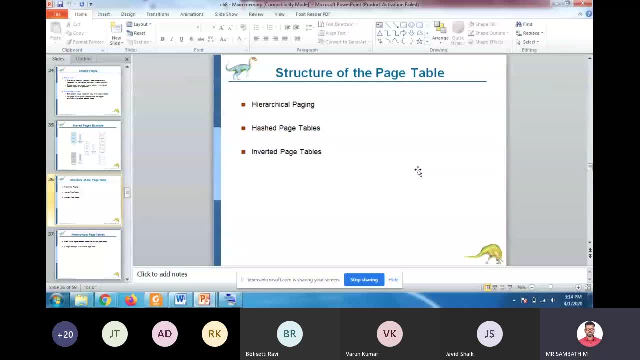 This page table is nothing but whatever we have discussed previously in the previous slides. So this one is the page table. So how you are going to maintain that page table is these three types. So the first one is hierarchical paging. In the hierarchical paging what happens is: this is your main memory. 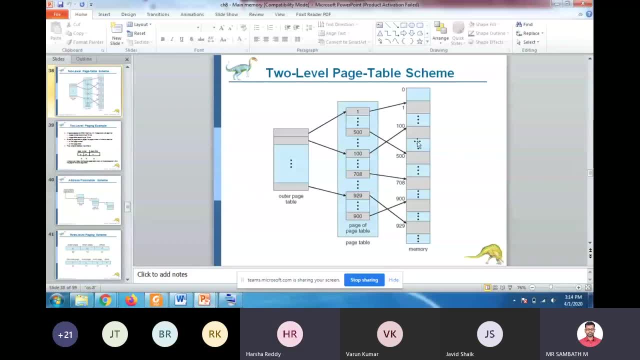 For this main memory, we are creating a page table. Then again, for this page table, we are creating another page table. Why? Because, for example, if this main memory is, for example, if you have 1000 locations, This one page table is enough. 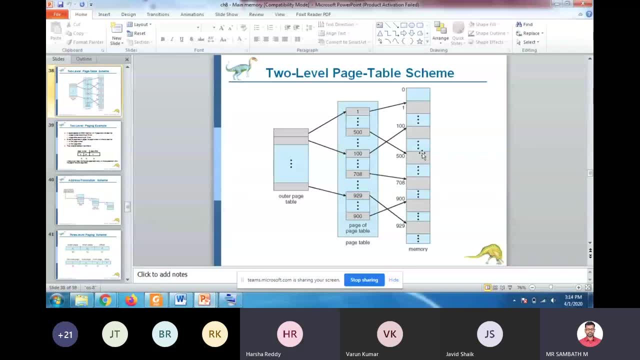 For example, if the main memory is having like 1 lakh location or 1 crore locations, Then what will happen? if you make a page table for this main memory here, This page table will become very, very large, Like this page table will become having 1 lakh entries. 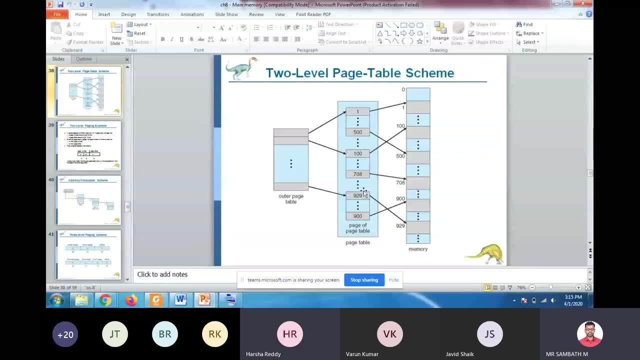 Then what will happen is: this is just like. this is the content of the book and this is the index page of the book. Imagine the index page of the book goes for 100 pages. Then what will happen? Again, it will be very difficult to find in the index. 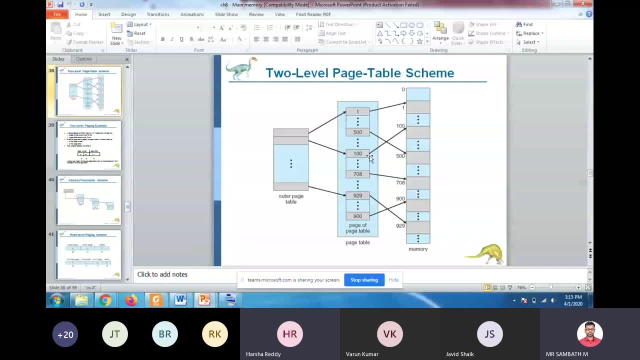 So what they will do is, again, they will make index for this index page. So that is what hierarchical paging. This is the first index For this index. again they will make this outer page index. So this concept is called two level paging. So you have two level page tables. 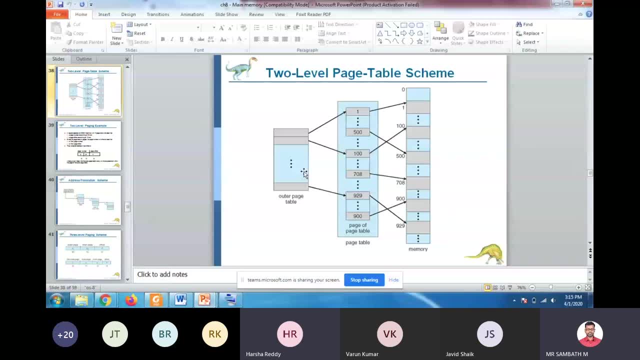 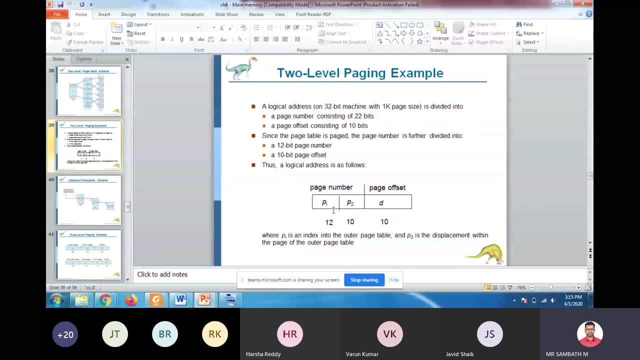 The next topic is how the address translation takes place. here is: This is the page number. Here the page number is divided into p1 and p2.. Then the offset is: as you should know, Previously we have only p and d. Here it is divided into p1 and p2.. 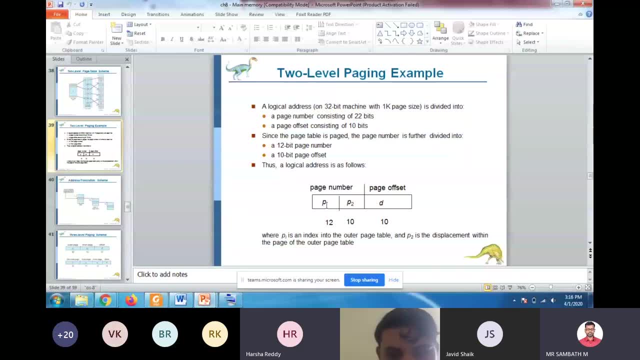 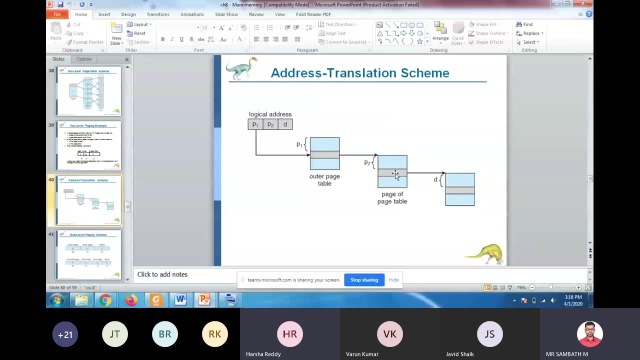 This p2 is the first page table and p1 is the outer page table. So first take this p1., Go to the outer page table, Take this entry, Then take this p2. And go to the other next page table And then again go to the main member. 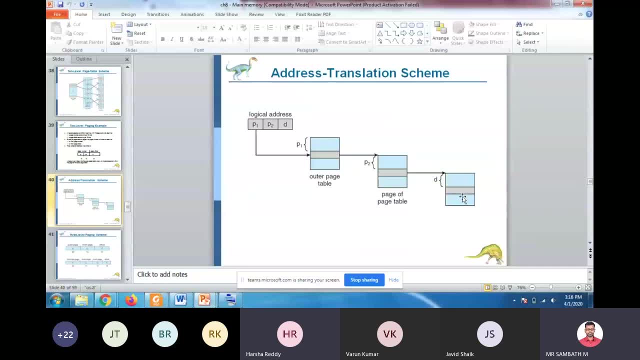 p1, p2, p3. Those numbers. The next one is hashed page table. So already you studied about hashing, What is hashing in data structures. So here we have the logical address p and d. So this page number is applied with some hash function. 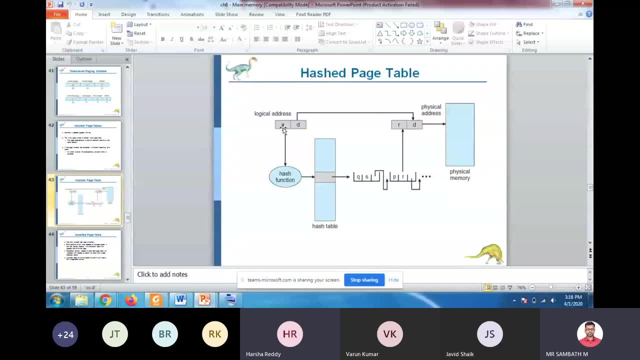 For example, the page number is 100.. The 100 hash 10.. Hash 10 is the hash function. Hash is nothing but, like we can say, it is a modulo function. So 100 mod 10, how much you will get 100.. 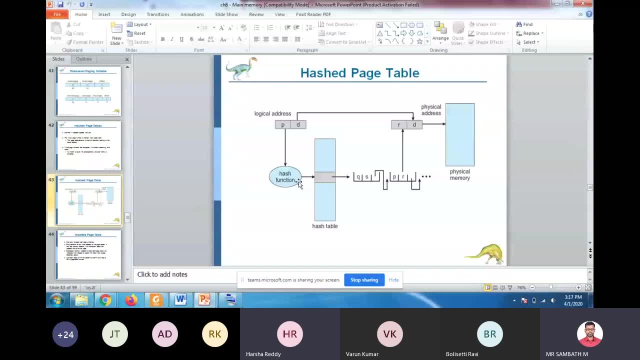 So you will get 100.. Sorry, 100 mod 10, you will get 10.. So it will go to the index location 10.. And then it will take the data Whatever available here, And then it will take this entry And then it will combine this. 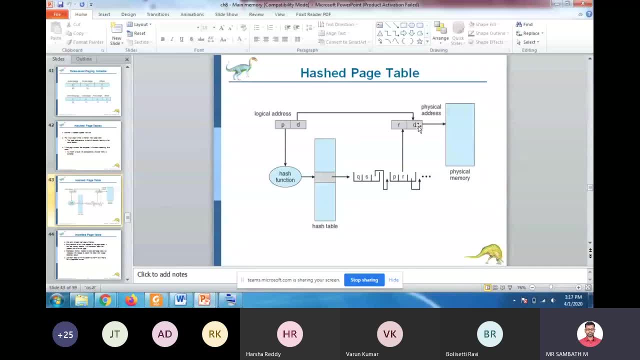 And then it will generate the physical address. This is the linked list which is attached to this entry. This is what hashed page table is. Take the page number, Apply the hash function, You will get some value And go to that index and get the corresponding frame number. 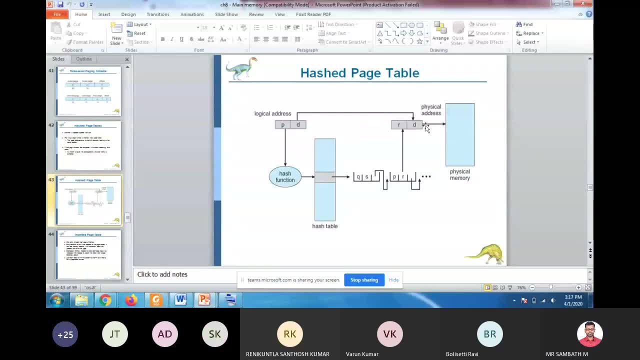 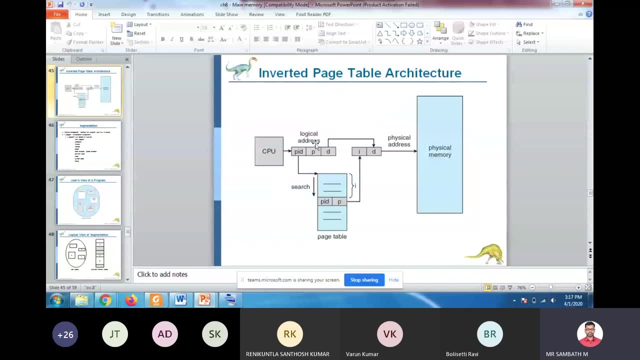 And attach it And then generate the physical address. The next one is inverted page table. In inverted page table, what happens is The CPU will generate logical address Which is combined with something called process ID. You know what is process ID? Each and every process has its own number. 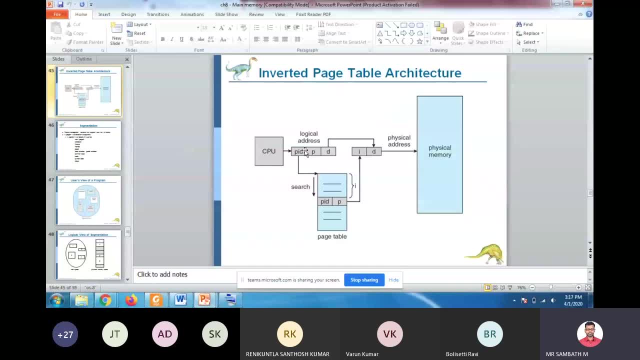 That is a unique number That is called process ID, PID, Which is combined with this logical address: Now this process ID and then page number. Both are used to find out an index into this page table And then take that entry And then combine with this as usual procedure. 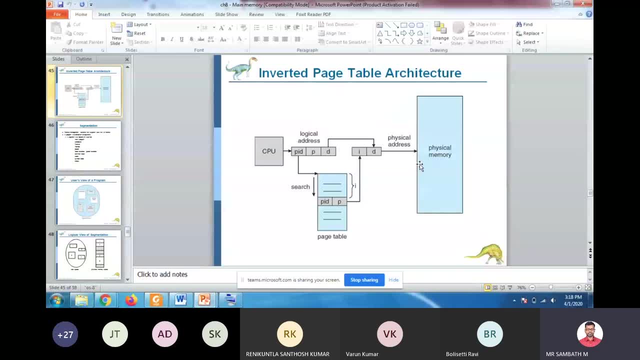 And then it generates the physical address. So that is the inverted page table. The value difference is combined with process ID. That is the only difference. The other concepts are same. So next we will move on to a concept called segmentation. In general, what we have seen is paging. 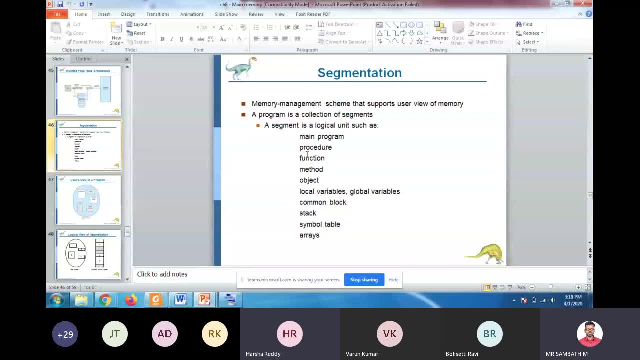 Now what you are going to see is segmentation. The main difference between paging and segmentation is In paging, all the pages are of equal size. For example, 100 KB page means all the pages will be 100 KB. This is also like pages. 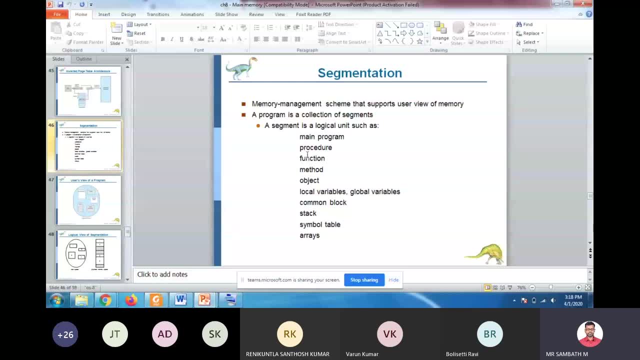 But the pages will not be of equal size. One page may be 100 KB, Another page may be 350 KB, Another page may be 500 KB. So it goes like this, Then how this segmentation works, For example, if you take a program: 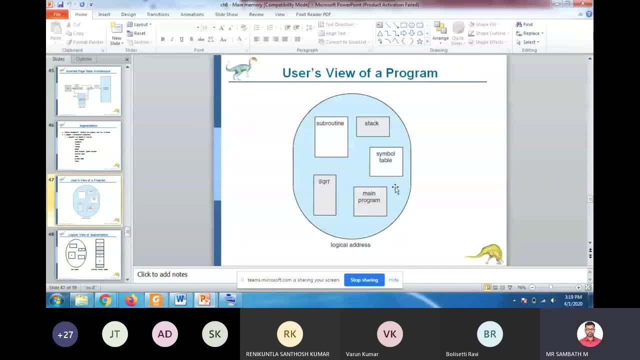 In your program you may have all this. You have the subprotein. Subprotein is like a function, Then square root is another function, Then you have main program, Then symbol table, Then you have stack. So your program is a combination of all these blocks. 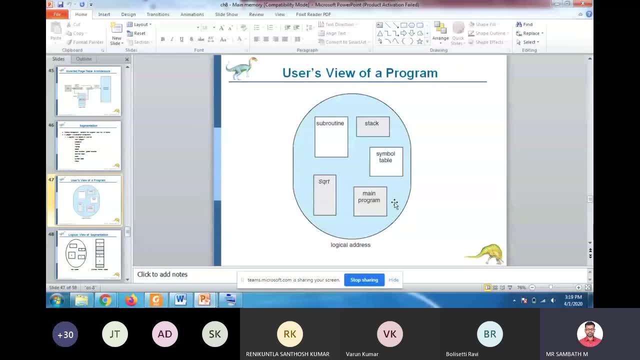 So, according to these blocks, They are going to make the segments. See here, 1,2,3,4 segments are there, So these segments will be mapped into this, The physical memory, like this: 1,2,3,4.. 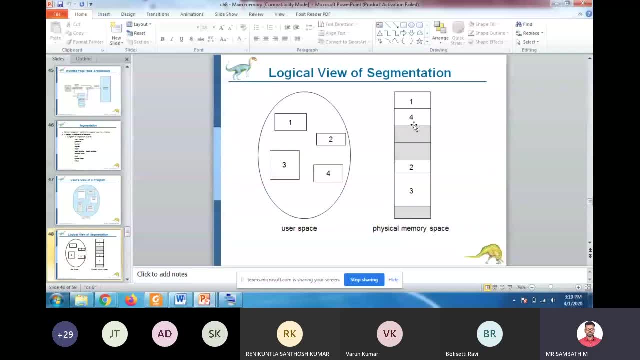 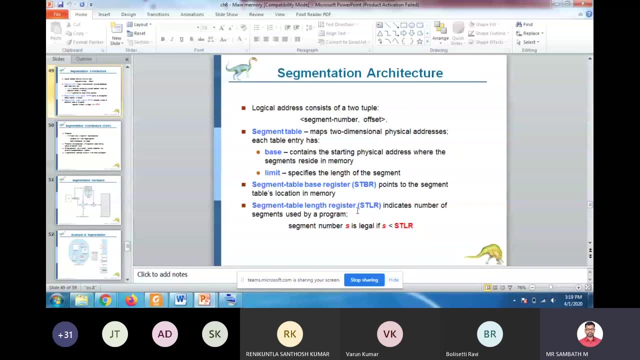 Now in page table we have page table base register And then page table length register. Similarly here we have segment table base register And segment table length register. That is STBR, STLR Base register indicates the base address of the segment. 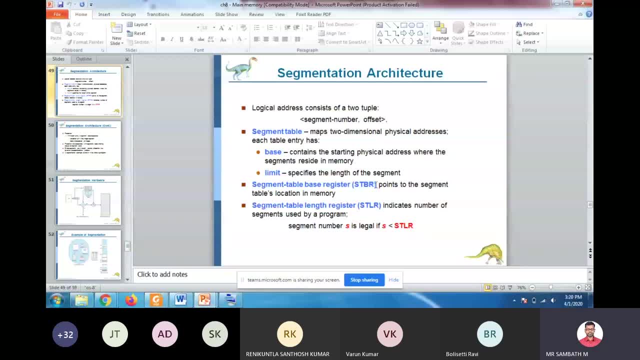 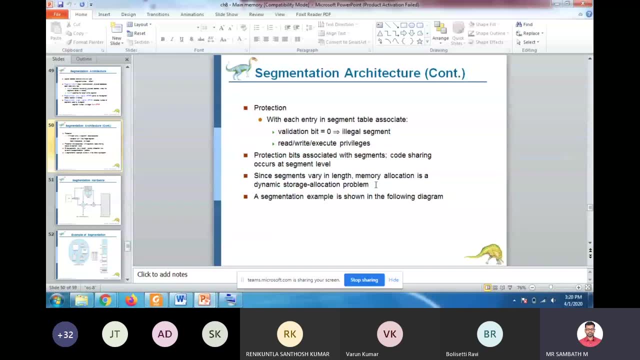 And the length register indicates The limit of the segment. Now how this segmentation works is like this: The CPU will generate this address, There is a segment number, Then displacement, Like as usual in your paging, And here there is a checking mechanism. 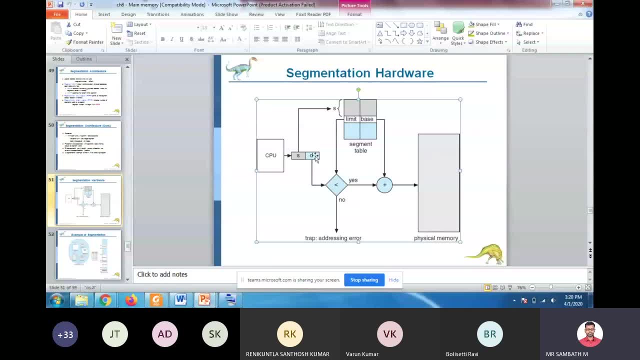 That is, this displacement is less than this, The limit allotted to that segment. Only if it is there, Then it will proceed with the addition operation Like conversion operation. If it is not within the limit, Then it will not do this addition operation. 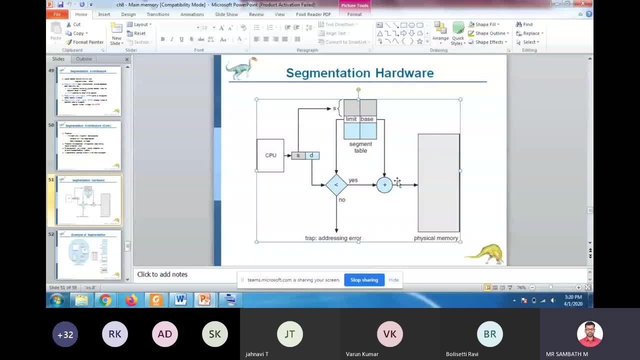 It will give you error. Take this segment number And go here And take this limit. This is the base address And this is the limit. And check. the limit is within Check. this displacement is less than this limit. If it is so, you proceed. 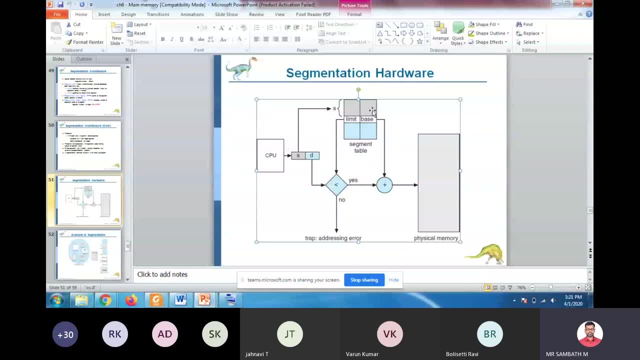 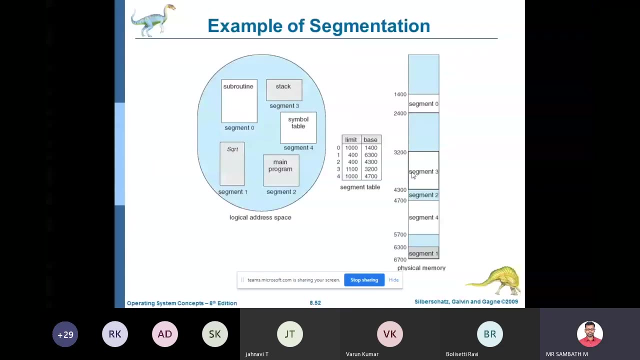 And take the base address And add with this And generate the physical address. Now this is an example. See here there are 5 segments: Segment 0, 1, 2, 3, 4.. Now how this segments are mapped into the physical memory. 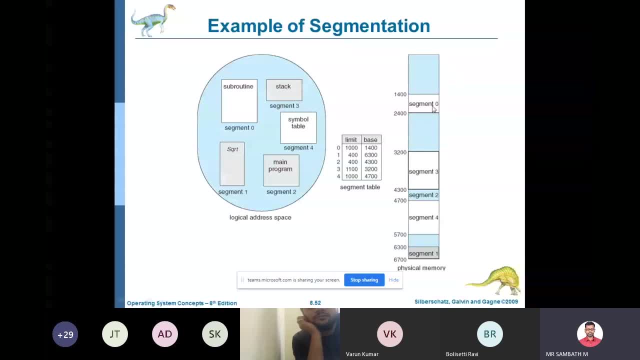 So there is a segment table here. See here, Segment 0.. The base is 1400.. Limit is 1000.. Now this is going to map like this: See here: 1400, starting segment 0.. Till what? 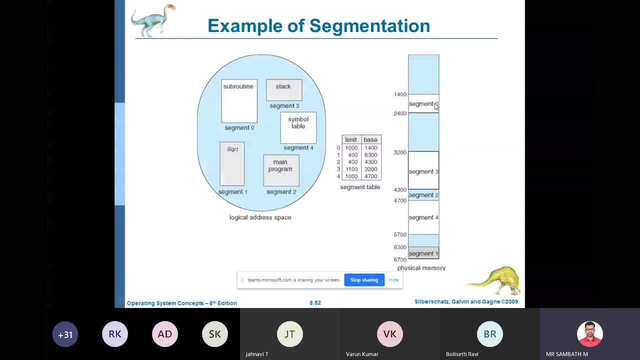 2400.. So the limit is 1000.. So 1400 plus 1000, you will get 2400.. So that is what this indicates. Similarly, you can look for other segments also. Segment 1. Base address: 6300.. 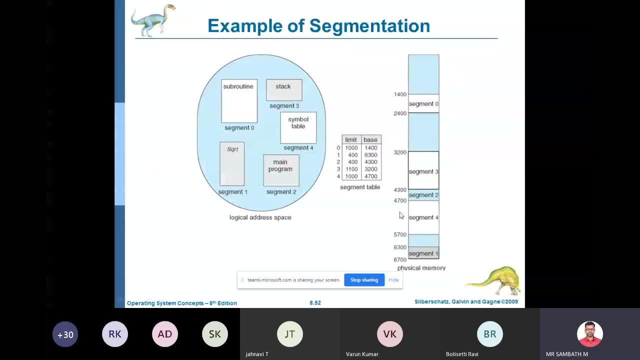 See here: 6300.. Limit is 400.. So plus 400.. 6700 is 6400.. 6700 is segment 1.. Then segment 2.. 4300 plus 400. 4700.. So this is how the blocks are mapped into the physical memory according to this segment table. 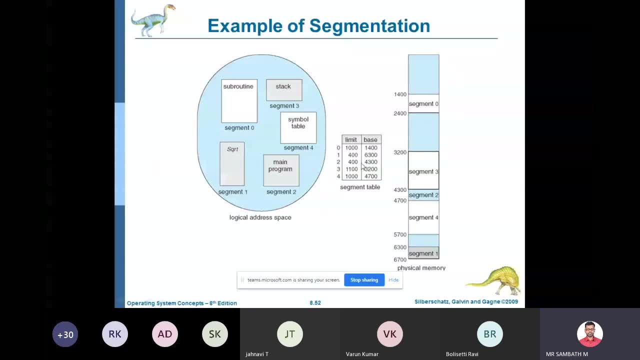 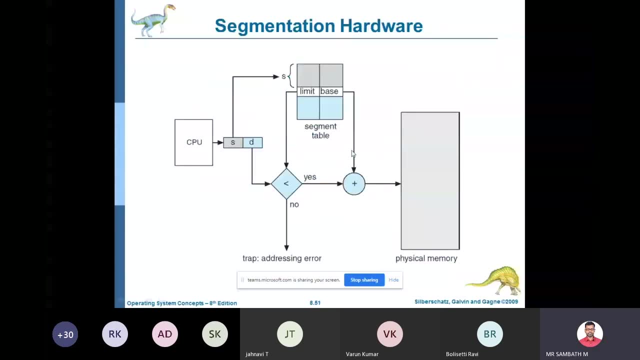 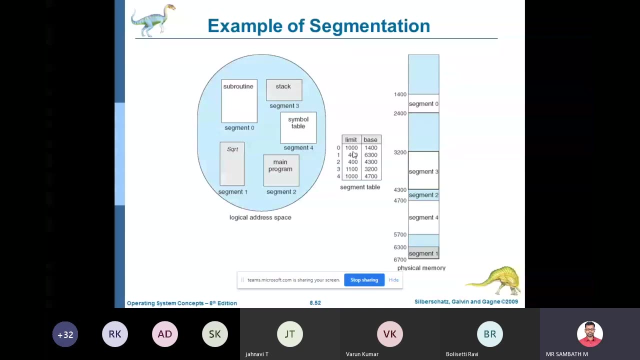 Now what happens is when I look at this previous diagram, See, this displacement should be less than this limit value. This displacement is greater than this limit, then it will give you an error, That is, you are not within that segment. The address goes out of the segment. 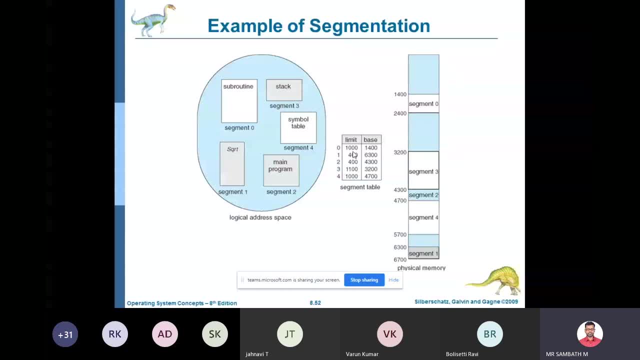 So it will issue an error. So this is the segmentation process. So paging is of equal size to blocks And segmentation is for different sizes of blocks. Okay, Otherwise, all the mapping mechanism, everything is same, Okay. So with this, this chapter is over. 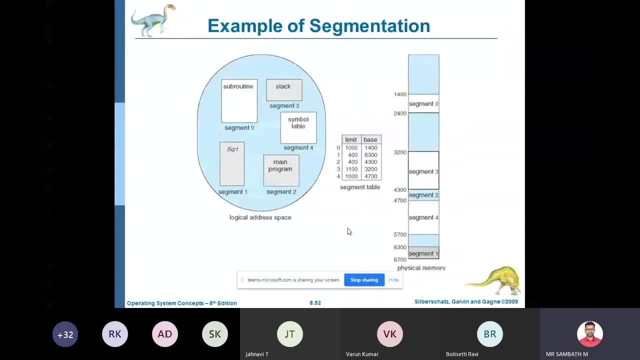 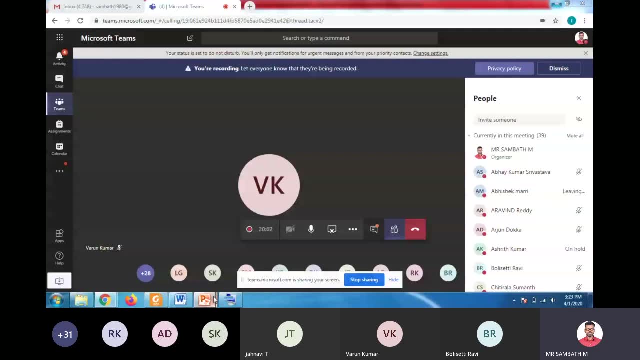 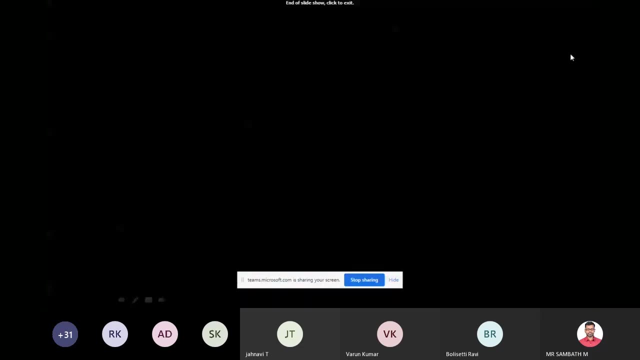 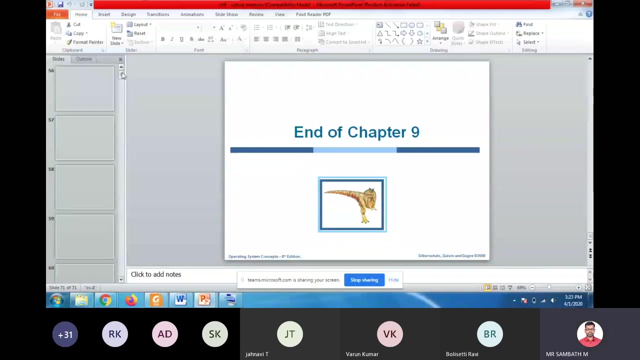 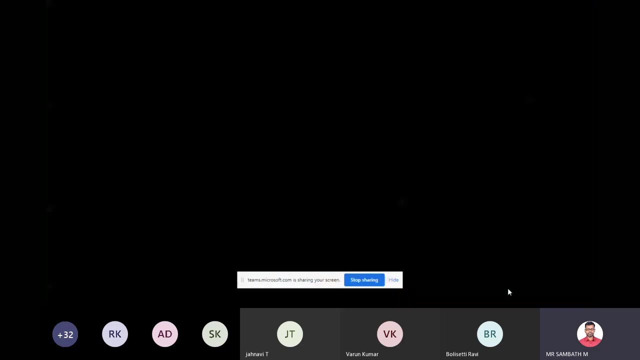 The next one, we will move on to the next chapter, That is the ninth chapter. That is the virtual memory. So what do you mean by virtual memory? One second? So virtual memory is like the ability to address more than the address which is available physically. 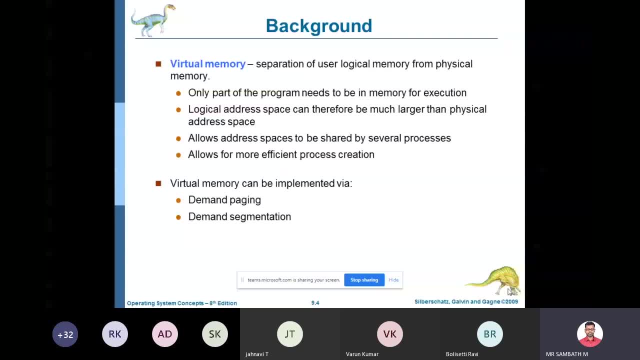 Okay. For example, in your physical memory is like you have only 4 GB, The CPU is able to generate the addresses, which is more than 4 GB Like it may generate. 4 GB means you can generate like only within, for example, 4000.. 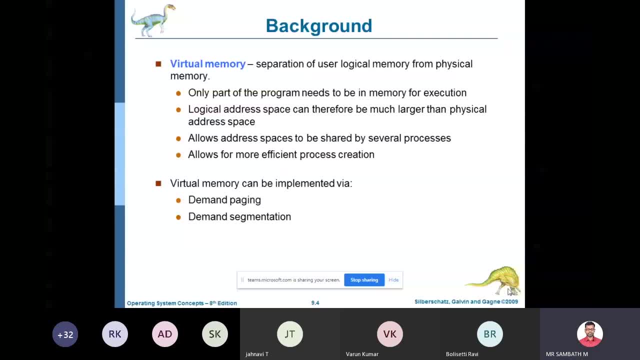 But the CPU may generate address which is more than 4000, also like 8000. Then in that case there should be some mapping mechanism to convert that virtual memory into physical memory. Okay, So that is what we are going to see here. 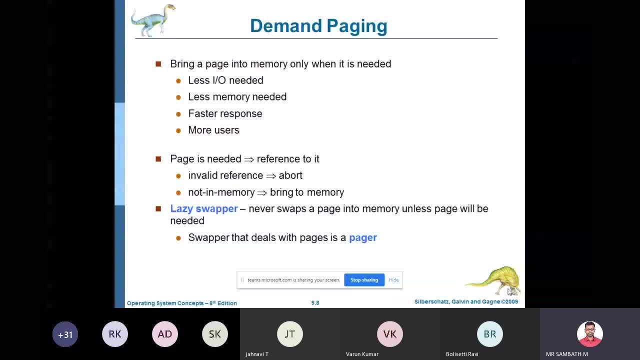 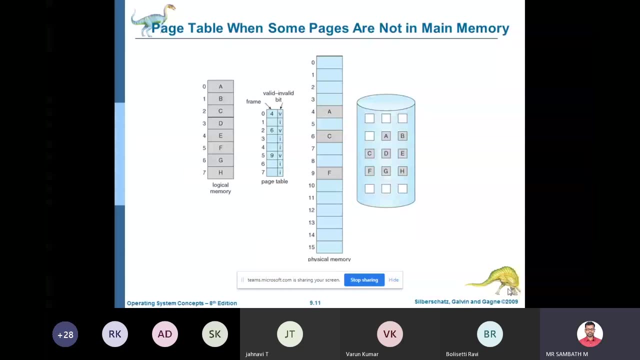 How the virtual memory works. So you will see what is demand paging. So this is related to the virtual memory concept: Paging. you know already What do you mean by demand paging. Whenever the process needs a page, the page will be bought into the primary memory. 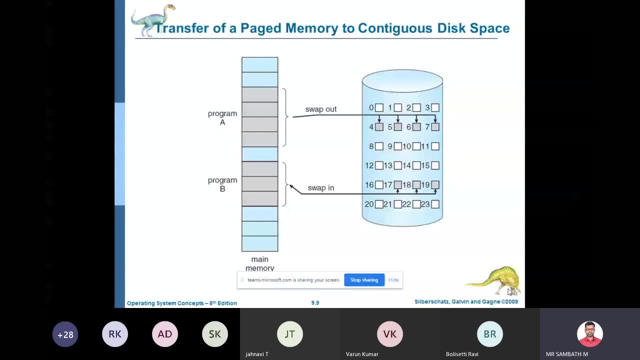 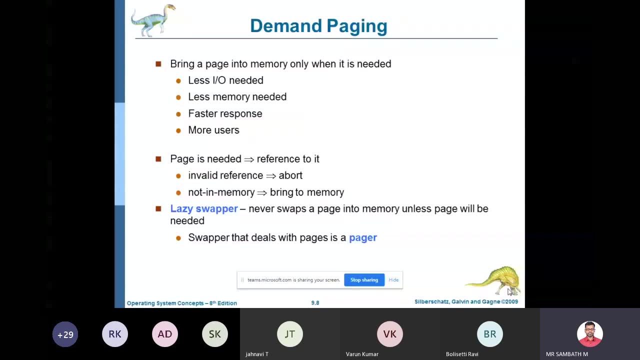 That is called demand paging. actually, Unless otherwise the page is needed, the page will not be bought into the memory. So whenever there is a demand for the page, the page will be bought into the main memory. That is called demand paging. Simple swap out procedure like program A is there and program B is there. 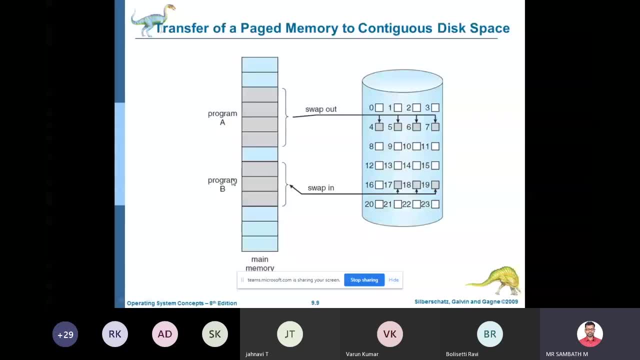 Program A is swapped out and program B is swapped into the main memory. So this is how the demand paging takes out the pages and put it in the hard disk And from the hard disk it will take the pages and put it into the memory. 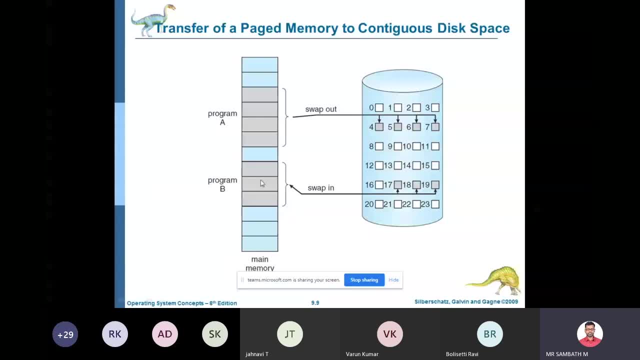 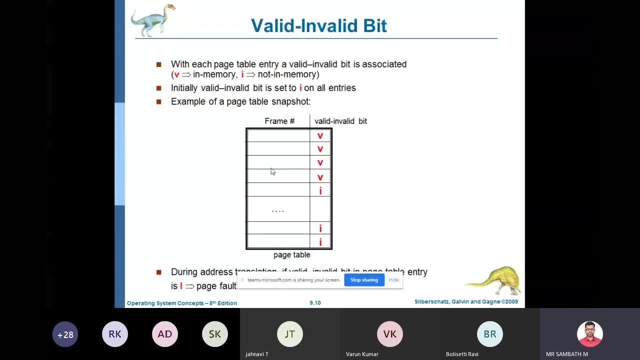 Now, what is this valid bit and invalid bit? For each and every page or frame- you can call it a frame in the main memory- For each and every frame you have a valid bit and invalid bit. B indicates the valid bit, I indicates it is invalid. 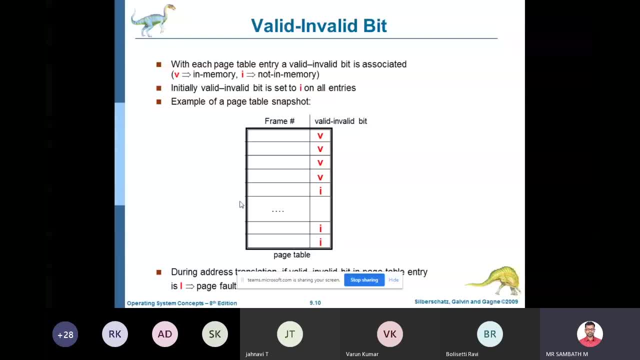 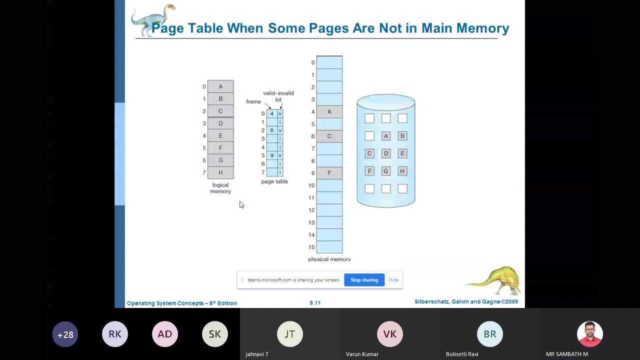 So it means that the page which is available in the memory is valid. B indicates I indicates the page is not valid. Some junk content is there in the memory. So that is what the valid and invalid bit. Whenever you are referring a page, if the page is available in the memory, that is called page hit. 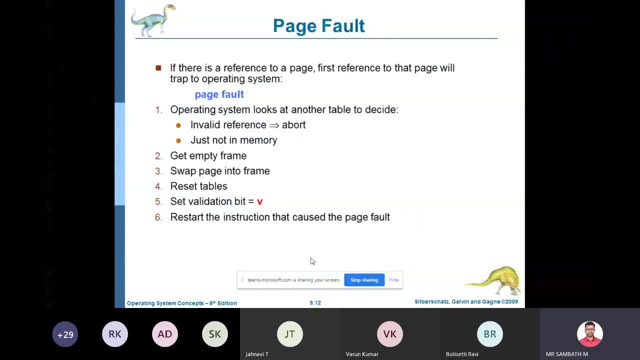 That is, page is available. If the page is not there in the memory, then that is called as page fault. If the required page is not available in the memory, that is called as page fault. Then how you are going to handle this page fault? 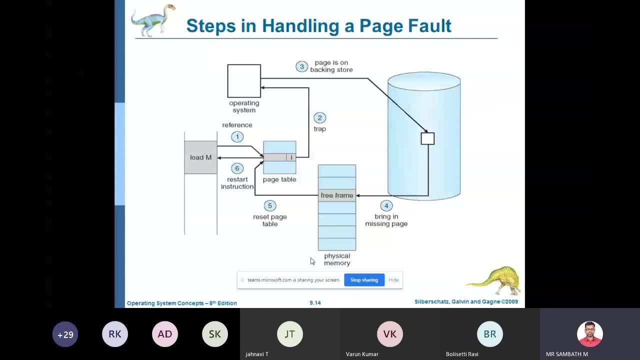 This is an important concept. Now, see here, They are trying to load some page That is called M Into this, But the page is not available here Because it indicates it is an invalid page. Then what happens? It will immediately send a request to the operating system to load the page. 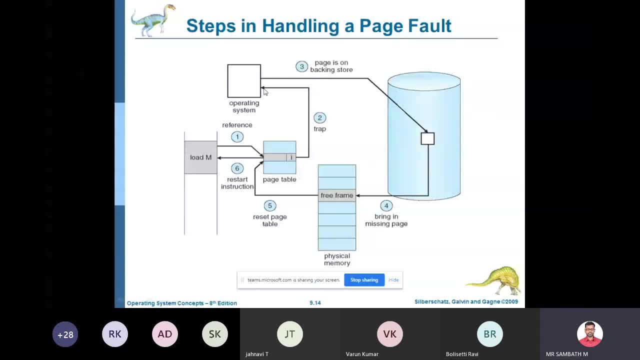 That is the second step. Then the operating system. what it does is: It will go to the backing store. Backing store is hard disk. It will go to the backing store, hard disk, And take the page, Bring in the missing page. 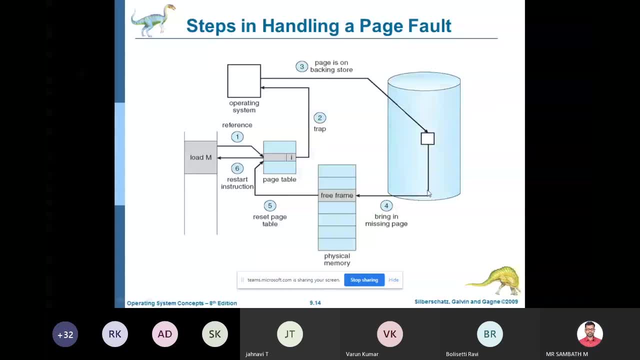 And load it into the physical memory, Okay. And then you update the page table. Here This page is available now. So you update the page table and make this bit as B And again you execute this instruction: load M. Now the page is available in the page table. 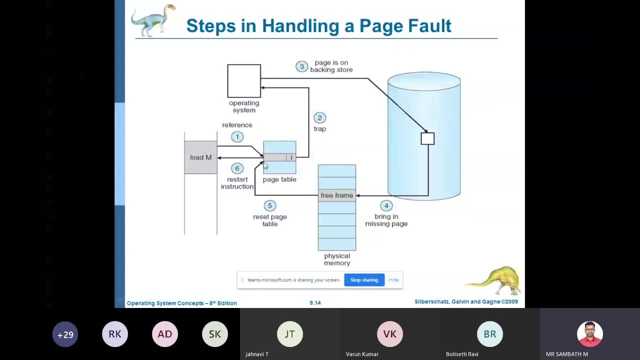 And it is available in the main. So this is what happens whenever there is a page fault, That is, whenever there is a missing page. So the instruction is referring this page. It is not available, It is invalid, So go to operating system. 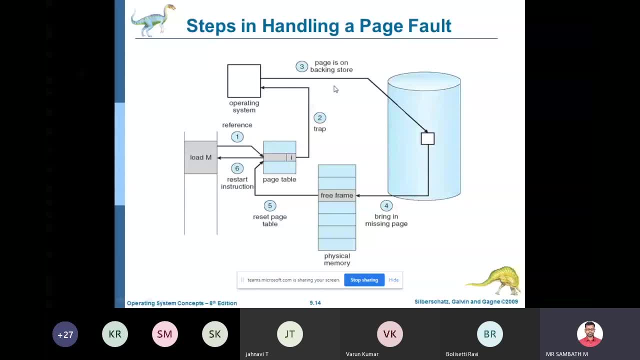 This operating system go to the hard disk, Brings the page And load it here And then update the table. also, It is a valid page. It will become B now Okay, So this is what the steps in handling the page fault. 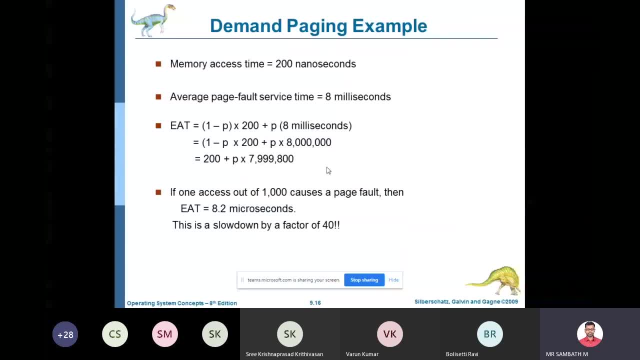 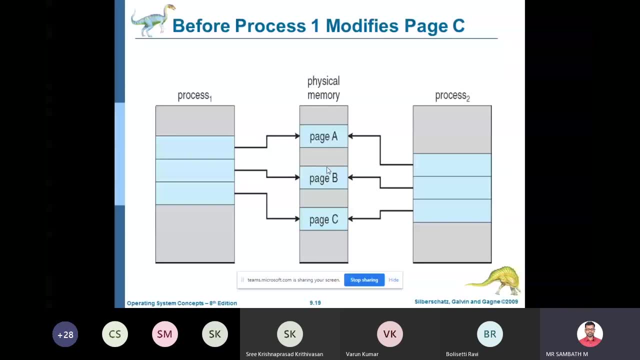 Now, what is copy and write? You already know that there are parent process and child process concept. Okay, You have like process 1 and process 2.. These two processes will be referring: page A, page B and page C. Okay, So see here, when you look at this diagram, 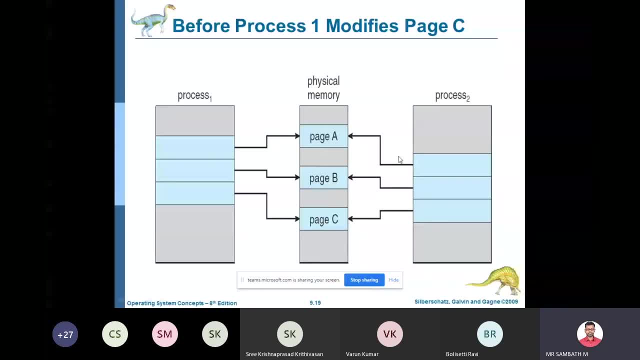 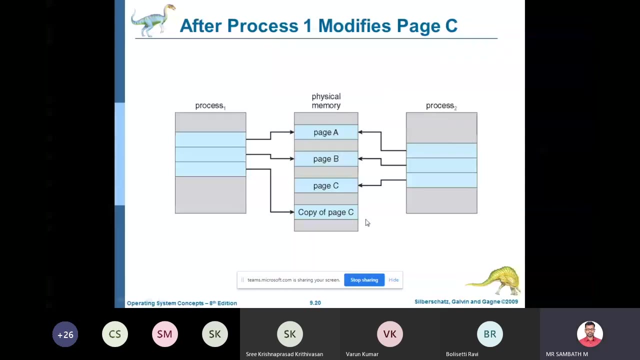 Page A is referred by process 1 as well as process 2.. Then, similarly, B is referred by both the process and C is referred by both the process. Okay, Now, whenever the process is making a change in any of the pages, Page C: 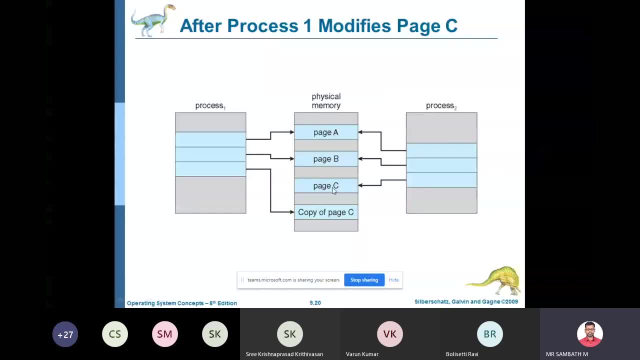 Then a copy of the page will be taken. See here, Page C is there still- And copy of this page C is taken, And then it will be referred by the process which is modified. This is what process called copy and write, Whenever the process is trying to write into the page. 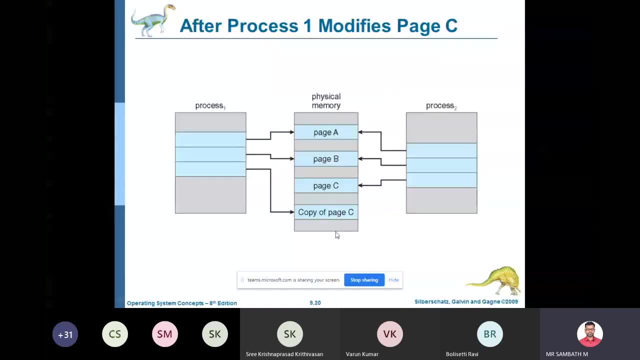 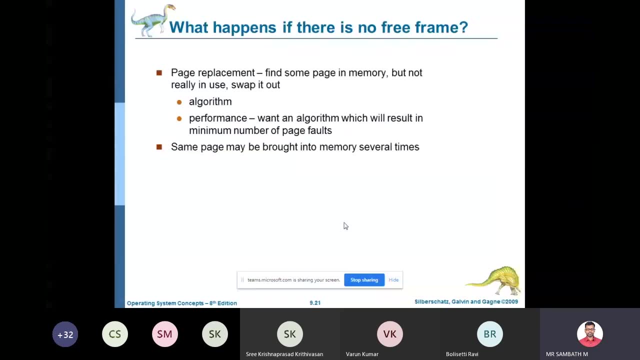 It will make a copy. So that is why it is called copy and write. Now imagine you are keep on loading the pages into the main memory. In main memory we will call it as frames. Okay, We are keep on loading the pages into the frames which is available in the main memory. 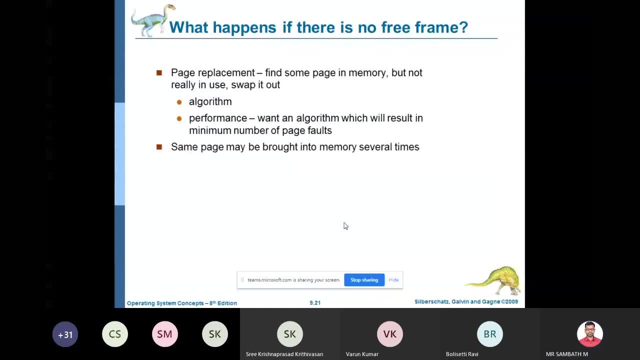 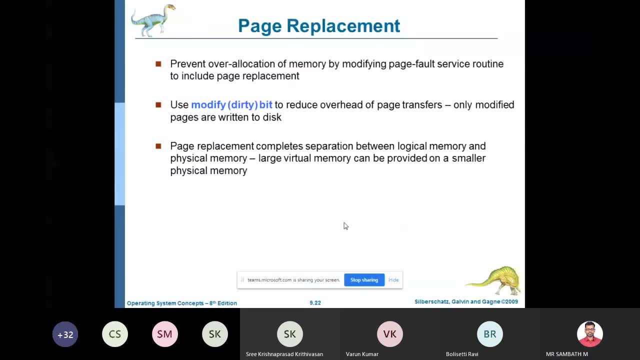 Now, once the main memory gets filled, Once the main memory gets filled, What you are going to do If the main memory is filled. You want to take the new page inside? Okay, Automatically. what you do now: You will replace the page which is already available in the main memory. 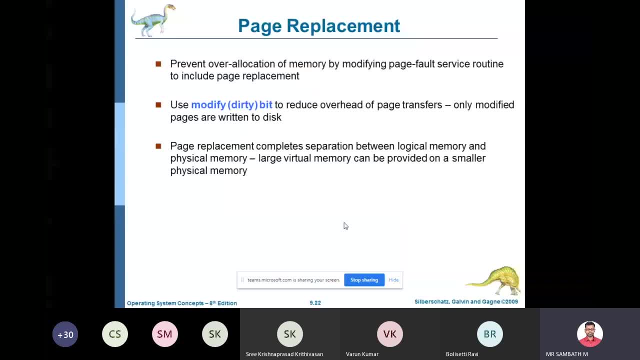 So that is what the usual process you will do. That is called as page replacement: Replace the page which is already available whenever there is no space in the main memory. So how you are Algorithms available to bring in the missing page, So you have to bring in the new pages. 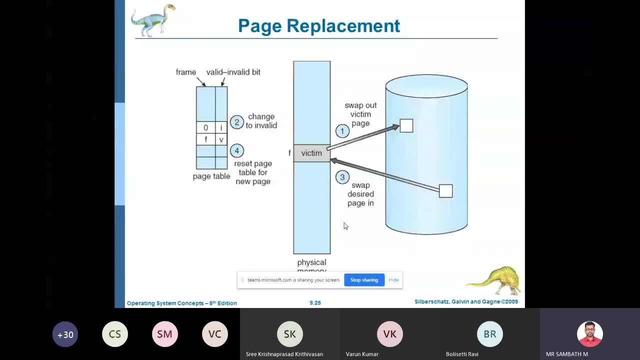 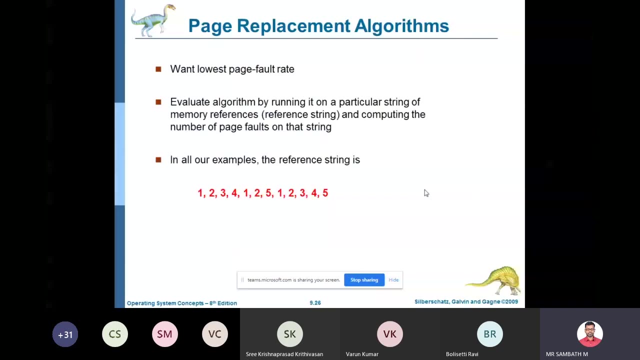 When the page is full. See here We are selecting the page- And then you remove that page and put it in the hard disk And again you bring the new page. So this page replacement. you cannot do just like that. There should be some procedure. 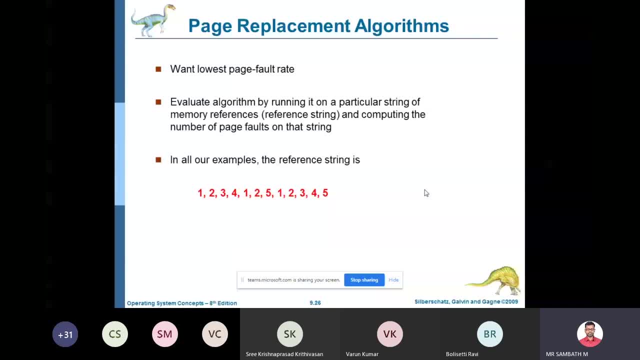 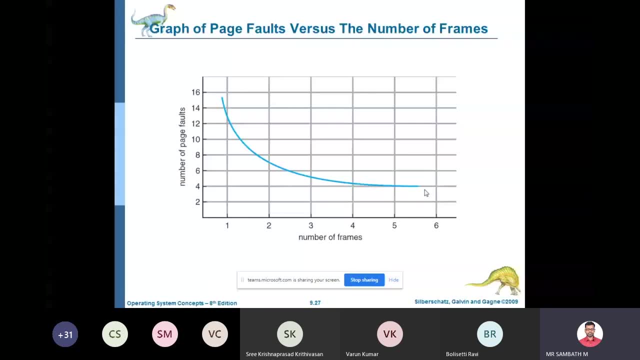 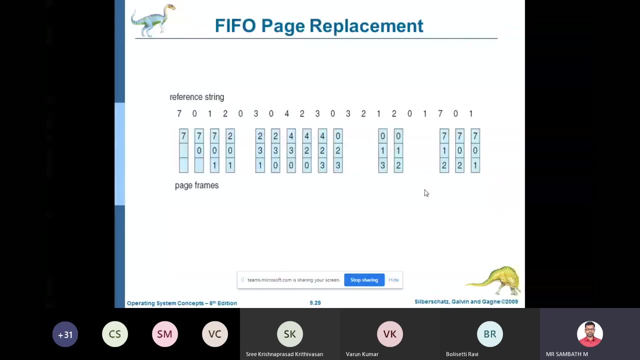 There should be some algorithms available. So there are some page replacement algorithms available. First, note down the algorithms. Whatever the algorithms available, First in, first out, There is a before Then optimal algorithm. Then, least recently used, There is a LRO algorithm. 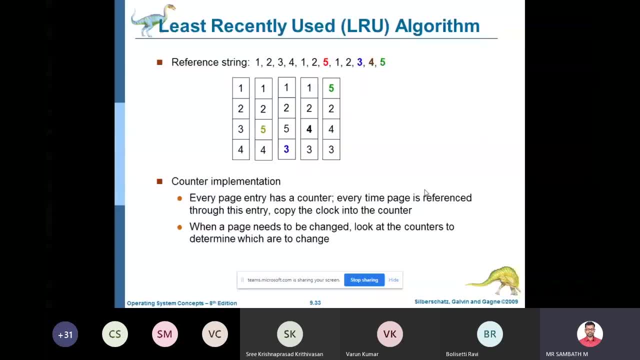 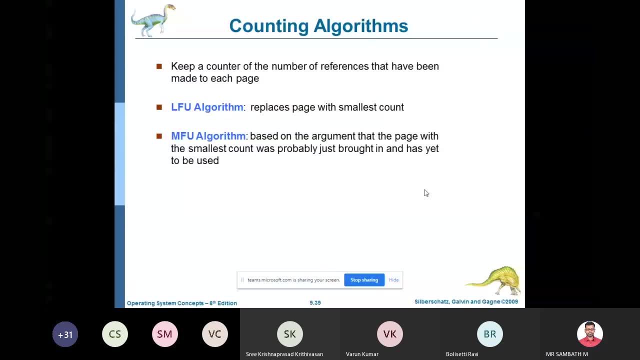 Then LRO approximation algorithms, Then counting algorithms. Okay, So you will see one by one. So what do you mean by before Before? everyone knows First in, First out, So whatever the page that comes first into the main memory, So what you are doing. 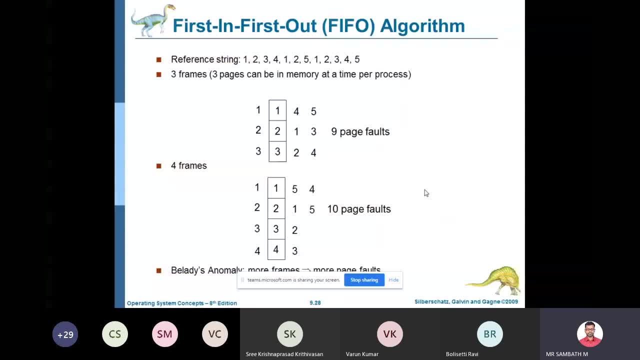 So it comes first into the main memory. That will be removed first When there is no space for the incoming pages. For example Here The page 123 is there already in the main memory. Now there is a new page. four is coming. 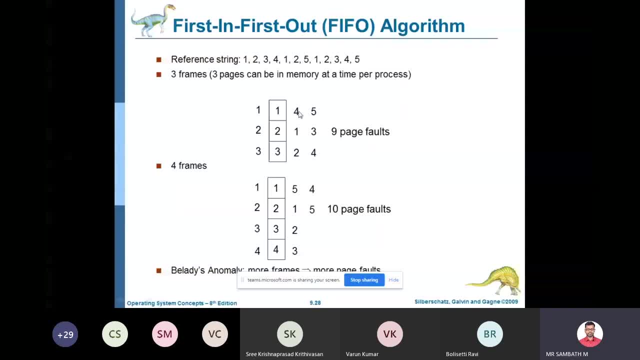 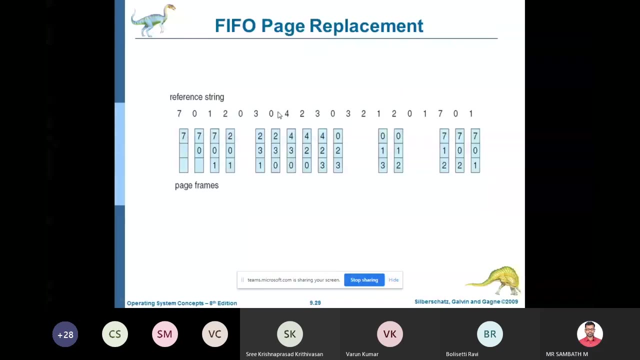 Now which one I will remove automatically, The one which comes first, That is the page number one. I will remove this page one first, And then I will put this page number four here. Okay, algorithms. you will see with an example here. now look at this diagram and this: 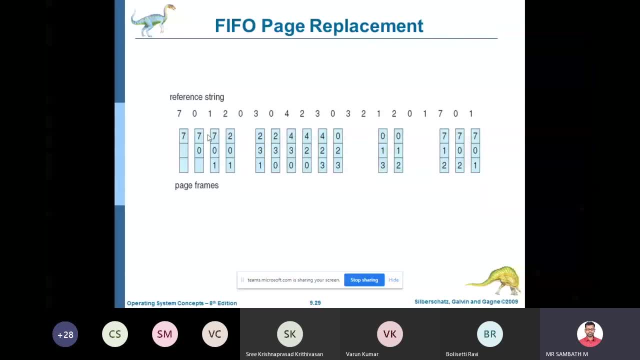 is the string. this number indicates the page numbers in the order which I am going to refer. okay, seven, I am going to refer first. that is a page seven. I am going a referring first, then I am loading zero, then I am loading one, then I am loading two. so it goes like this: so first seven is loaded, so initially. 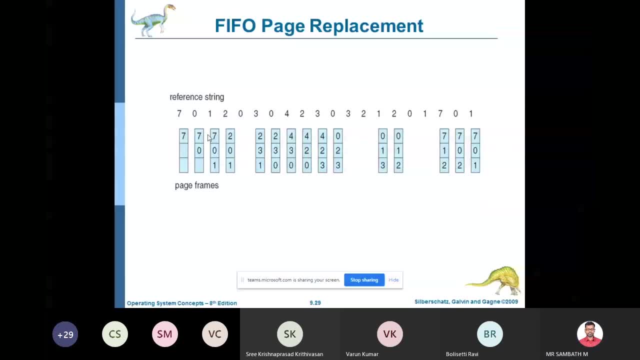 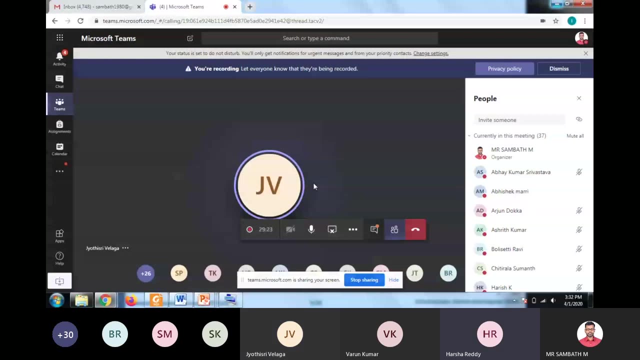 any doubts, sir, may be. someone is removing from the team, sir. yes, someone is removing from the game. the teams are members once, check the charts, that the charts are your wisdom, okay, so listen, this is very, very important topic. okay, now I am wrapping the page number seven. initially nothing. 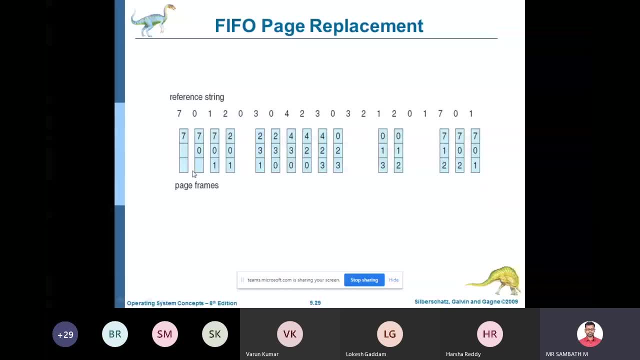 is there in the memory. there are only three oh, hmm, locations available in the memory. imagine: this is three frames, so i am loading seven, then i am loading zero, then i am loading one, so three pages are loaded now. now the memory is full. now i want to load this page number two. so which one i will remove first. 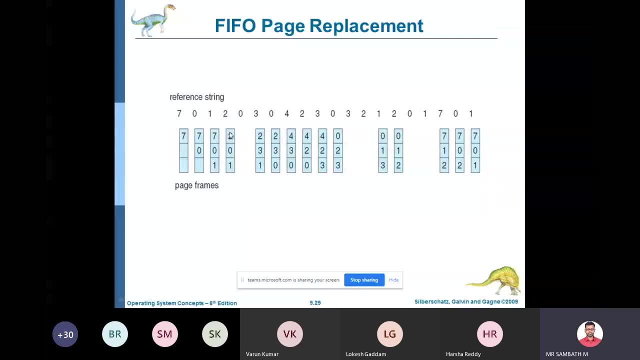 so automatically i will remove seven, because the seven is the one which came first. that is the first in, first out. so i am removing seven and i am loading two. is that clear? then next time i want to load page zero here you no need to load because zero is already there. is that clear? so that's why. 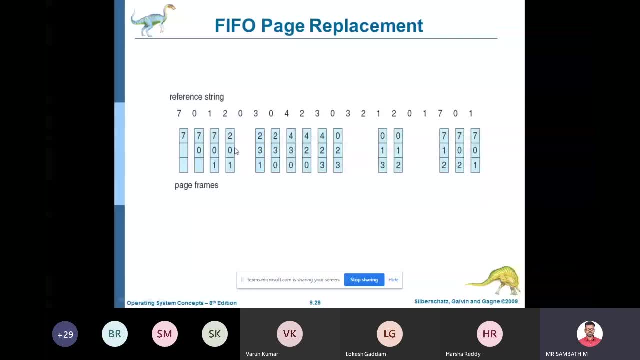 this place is empty now. next, i want to load the page three. now, see here, there is no page number three available. okay, but you need to remove some page here, so which one i will remove? zero is the one which came first, because the two is the one which came. 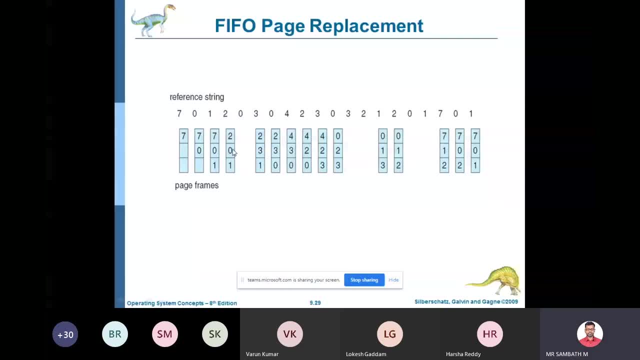 recently now. so i need to remove this zero. i need to load this. three here got the concept. next, zero i want to load, so i will remove this one, because the one is the one which came long back, so i will remove this. okay, so it goes like this: two, three, zero, then four is coming, then now i have to remove. 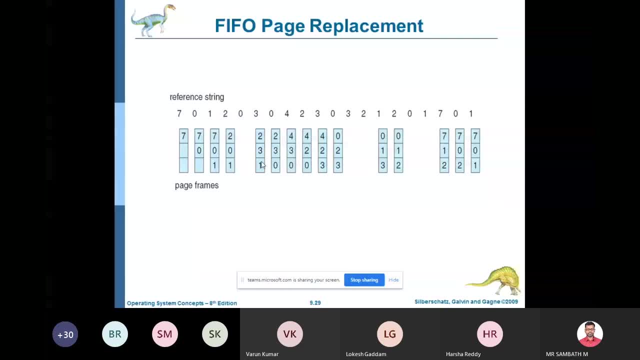 the page number one, zero, and then four is the number which came long back, so i know this is gonna be logo times over 28 piece. okay, and so now let's i go to my login box. now there, the account左 side. i got the information call. 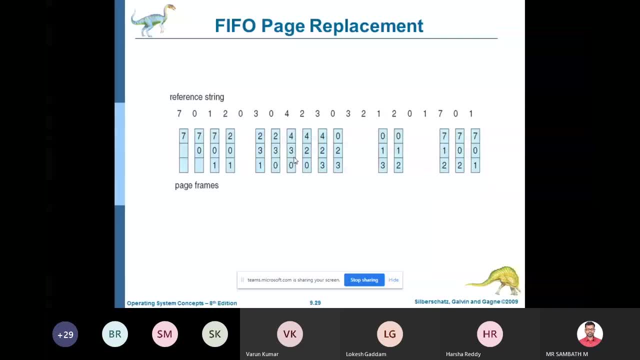 here you now. i need to do two things here. i will remove my username. please next time check it after you have done所以呢. the second one is what you now need to remember: mobile number two, three, four, five. then first thing you willие to do is just setup after. 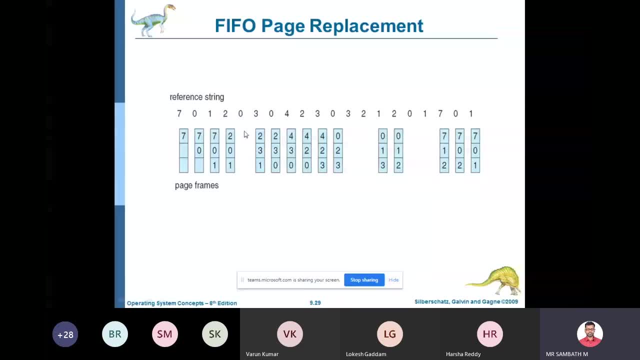 that i directly visit it like this and then click save and then click copy, and now here this place, there is no page fault because zero is already there. so no page fault. so four, five, six, seven, eight, nine, ten, eleven, twelve, thirteen, fourteen, fifteen page calls earlier. so this: 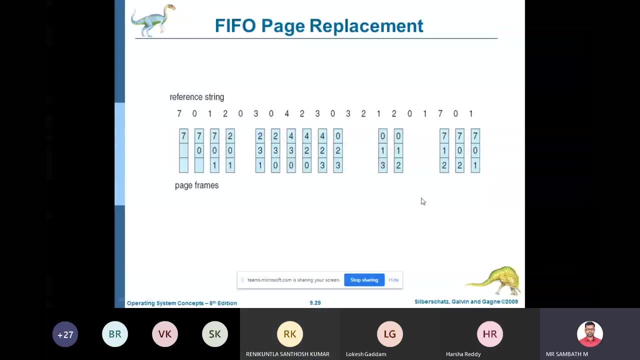 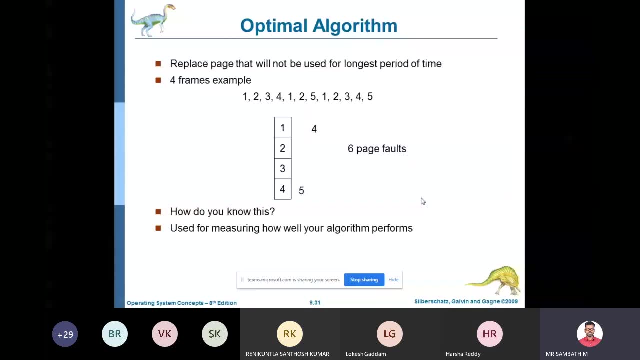 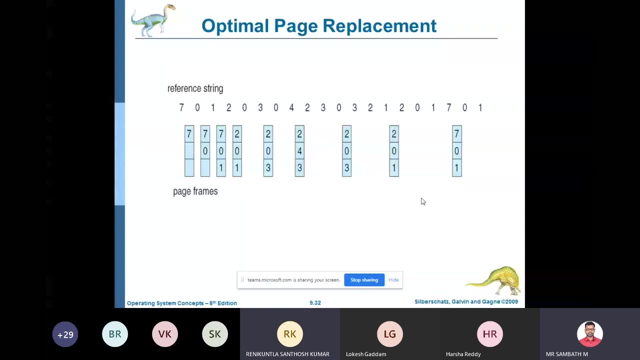 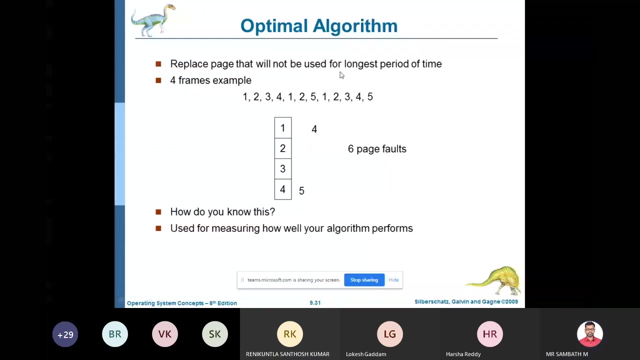 is how you have to calculate page fault. okay, so this is that before before algorithm. the next one, optimal algorithm. so optimal algorithm: replace the page that will not be used for longest period of time. see listen, that will not be used for longest period of time. it means that if you 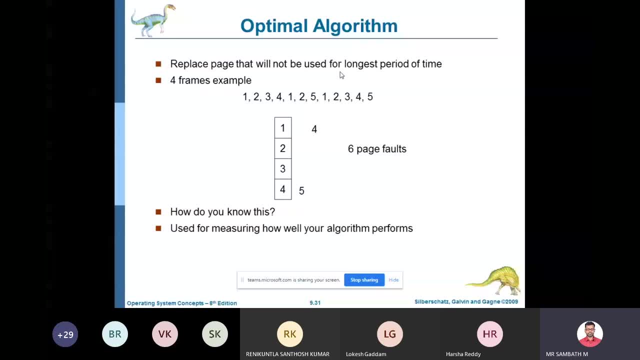 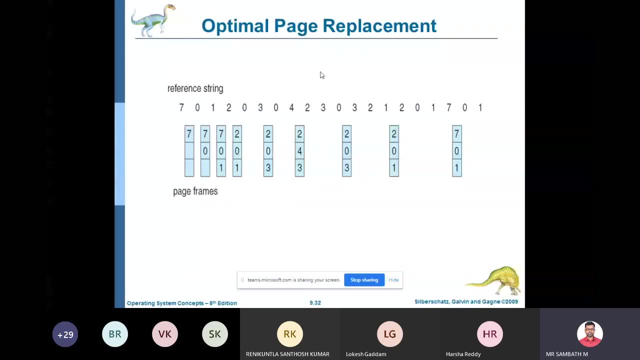 imagine that this page will not be used in future. then you can remove that page. that is called optimal page. so how do you know that this page will not be used used in the future? so you'll have to look at this reference string. see here: seven zero one. so 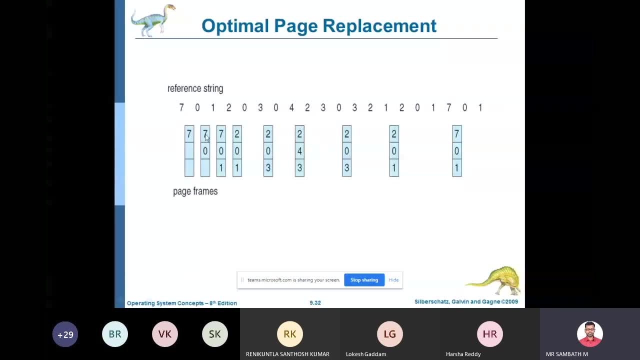 initially you have three page fall because the main memory is empty. no, so seven is loaded, then zero is loaded, then one is loaded. now it is full. now i want to load zero, so which one i will remove. you'll have to look at this feature, see here. look at all these numbers in the future reference. 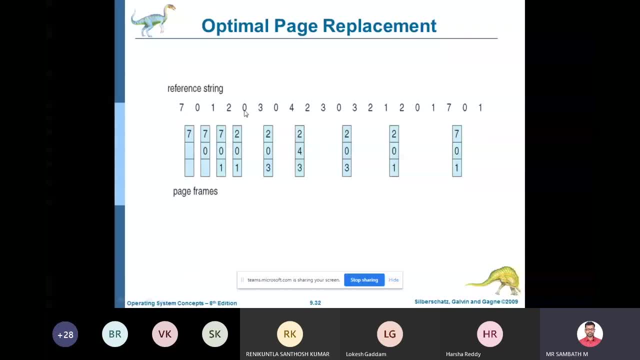 so zero is going to be used in the future. so zero is going to be used in the future, so zero is going to refer next time. so what i have to do? so don't remove zero. next three is going to refer. three is not there, so leave it. next again zero. next again four is not there. next two: three, zero three, two one. 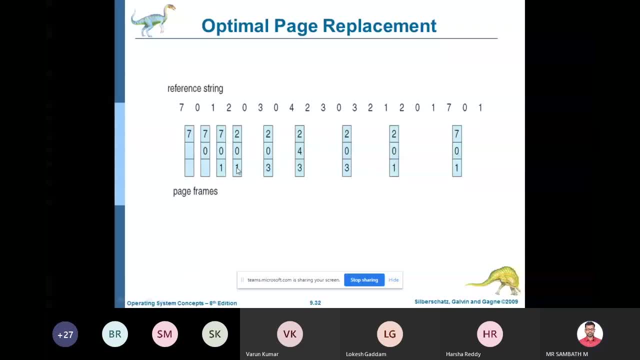 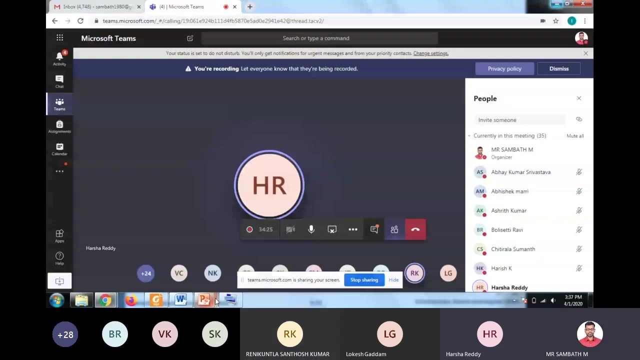 is going to be referred next time, so don't remove zero one. next two. zero one seven is going to be record after long time, so i will remember. but someone is playing, sir just. uh, who is that guy sir here? uh, just, it shows someone. sir me, i will remove him. 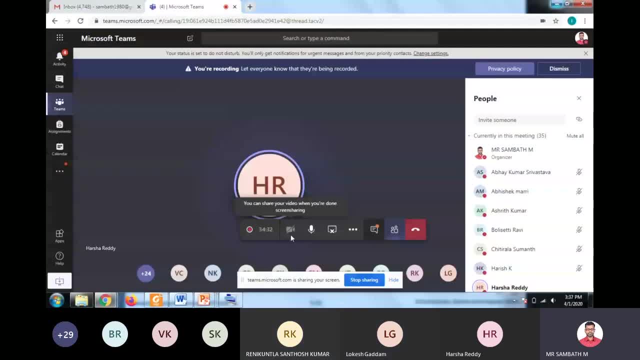 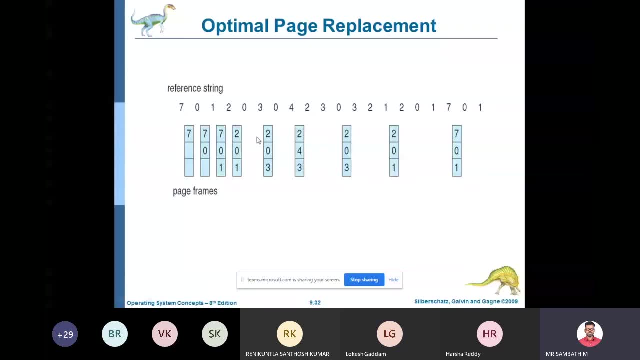 okay, okay. so here we'll have to look at the future reference here. now zero is there, so there is no page fall. next time three is coming. so after three, zero, four, two is going to be referred, so zero is there, and four is not there, and two is also going to be referred, so zero and two are the next. 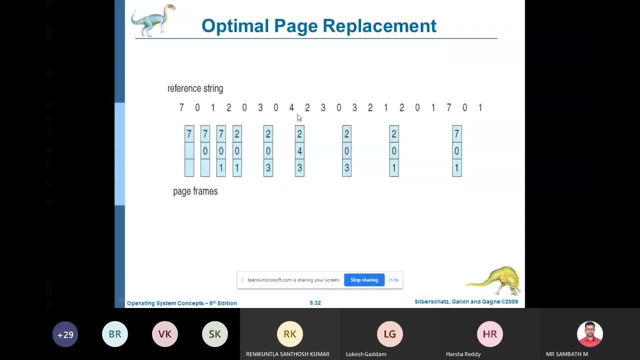 references, so which one? i will go going to remove one because one is not referred in the future, the near future, okay. so one is referred after long time, so i will remove one year and then i load this three year. so this is how you have to look at the future numbers and then remove the page which is not used for long time in the 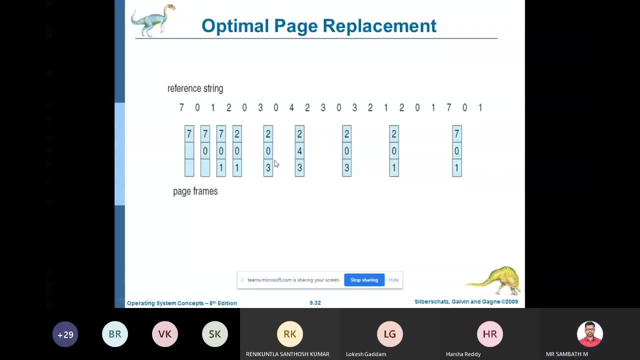 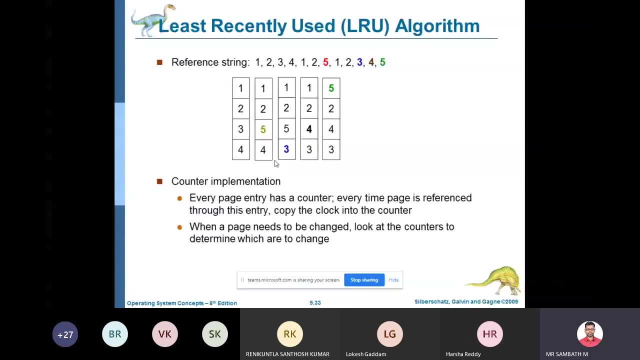 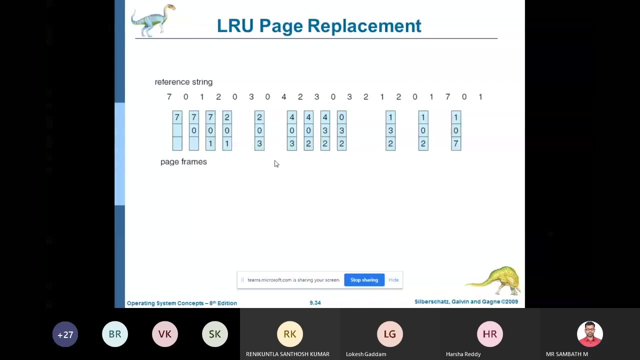 future. okay, that is optimal page replacement. next one: lru. lru is the just reverse of the previous page. so that is optimal. you will have to look. look at the back references now. see here: 7 0, 1. that is actually loaded now. 2 is coming now. go back and see. 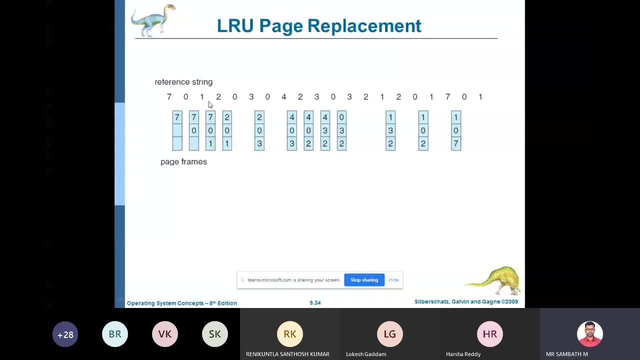 previously. 1 is referred, 0 is referred, so don't remove 1 and 0. so remove 7 and put the new page. got it. 0 is there, so no problem, next time 3. so when 3 comes, which one i will remove? don't remove 0, don't remove 2, because these two are recently referred, that is. that is what the 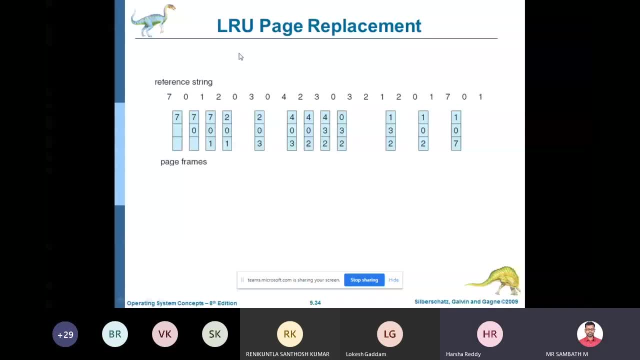 least recently used, so remove the page which is least recently used. don't remove the page which is recently used, which is recently used. 0 and 2 is recently used, so don't remove that. so remove any other page in this: 0, 7, 0, 1. okay, so 0, 2 i am not going to remove. i am going to remove 1. 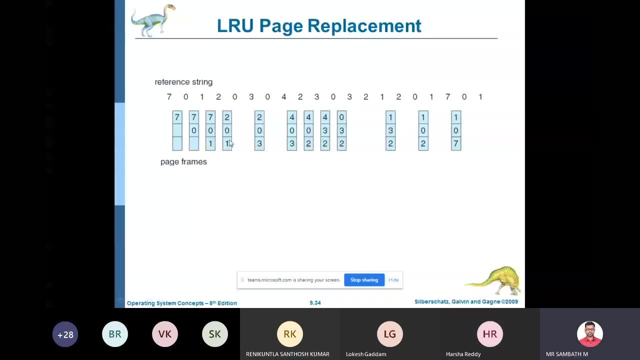 so i will remove 1. i will put this new page 3 here. okay, at the back, that is the past numbers, look back. okay, so that is a lru algorithm. so the next time 0, 0 is there, so next time 4 is coming. 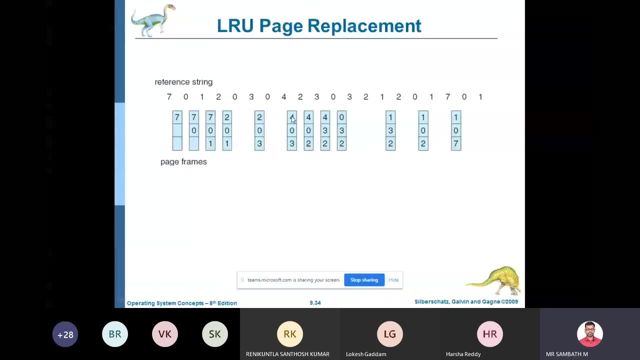 so when 4 is coming, there is no place. so i want to remove some page. so look back: 0, i should not remove. 3 i should not remove. so the 0 is there. 3 is there, only 2 i have to remove. okay, so this is. 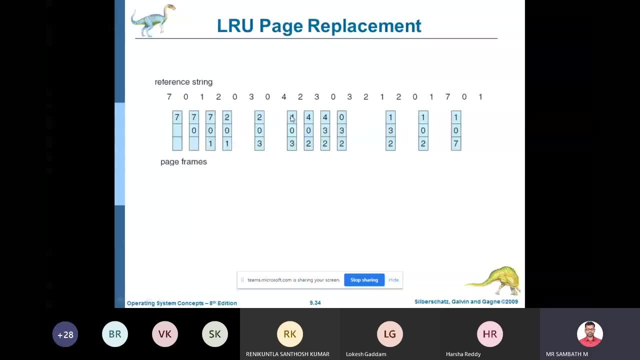 how it goes. so at last we can find out how many page calls are available. three, four, five, six, seven, eight, nine, 10, 11, 12 page calls are available so whenever the page is there already in the member. So don't draw the box here, Leave it empty. Whenever the page is not there, this one is not there here, So I will draw a page here and then I will put that page. So this is how you calculate the page number. 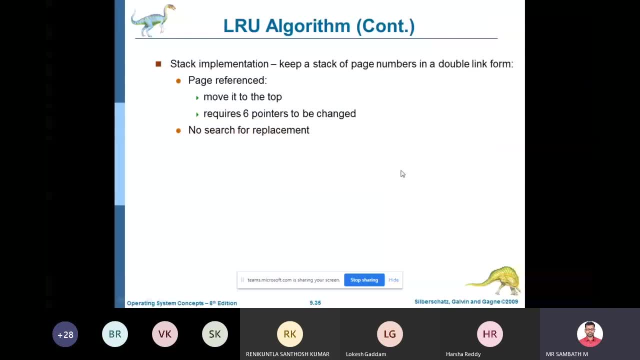 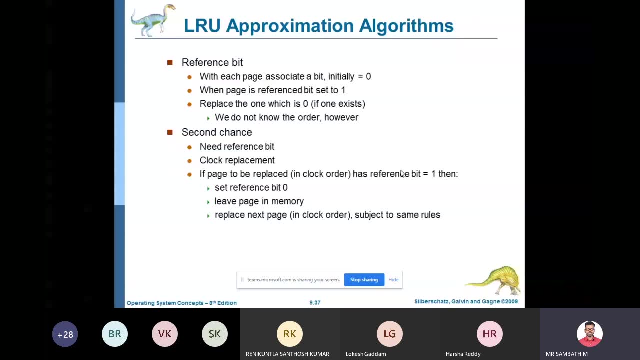 Okay, The next algorithm is LRU approximation algorithm. So this is derived from actually LRU algorithm. So there are two algorithms available. One is reference bit, The other one is second chance. This reference bit is like: with each page you attach a single bit. Okay, So that bit will indicate this is called reference bit. This bit will indicate whether the page is referred recently or not. 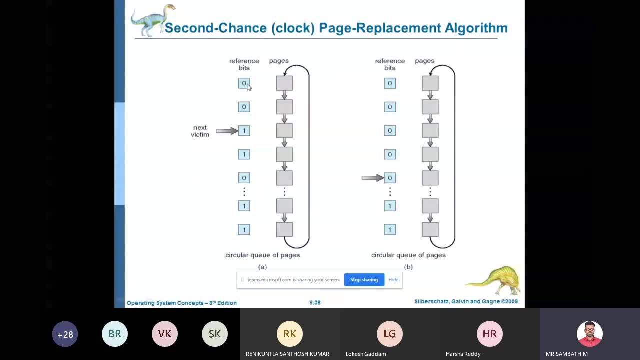 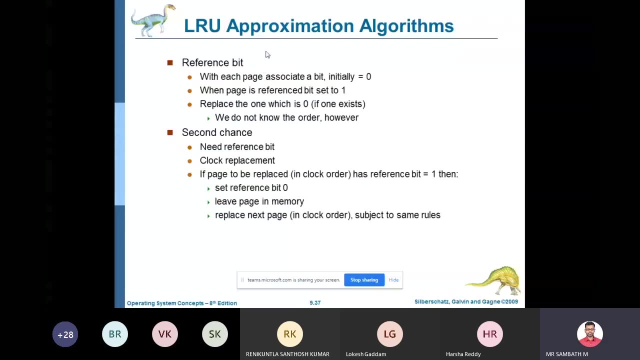 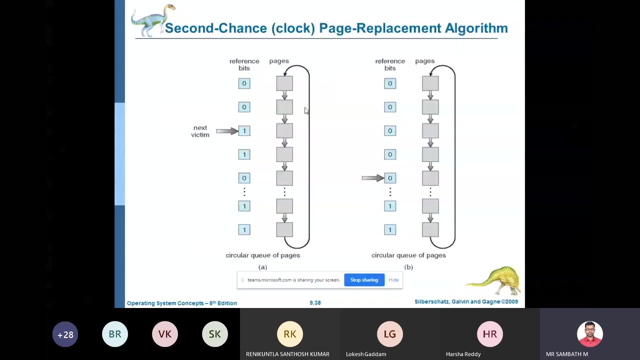 See here: if each bit associated with initially it is zero, when the page is referenced bit is set to one And the page is referenced, it will be set to one, Like this: In some pages it is said to have one, So it means that the page is referred recently. So don't remove that page. So which one I have to remove? 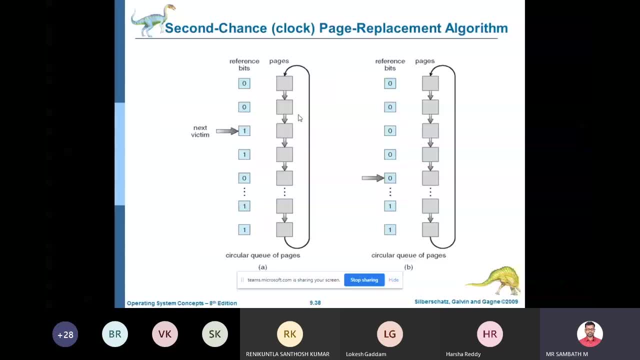 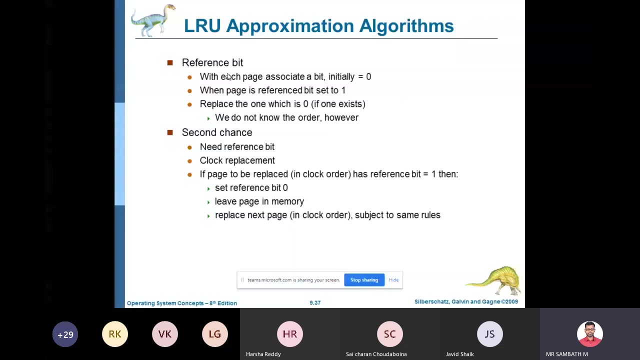 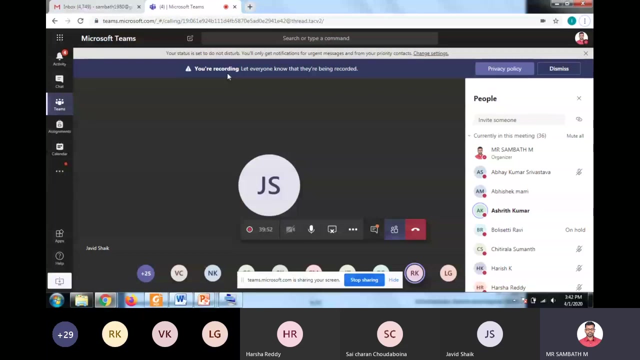 I have to remove this one, the page which is zero one second. all of you wait for two minutes. wait, wait, we will continue. continue, one second, wait. let me all of you mute your mic, please. yes, sir, wait, wait, let me finish. mute your mic. ok, so i will continue. 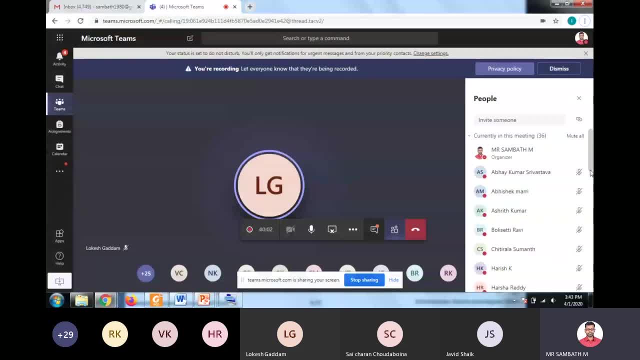 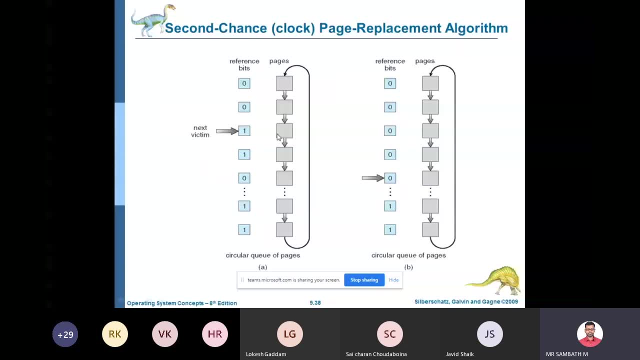 so lru approximation. there are two algorithms, i told you, reference bit and second chance. so reference bit will be initially zero. if the page is referred, that will be made as one. so when the new page comes, you remove the page which is having reference bit as zero. 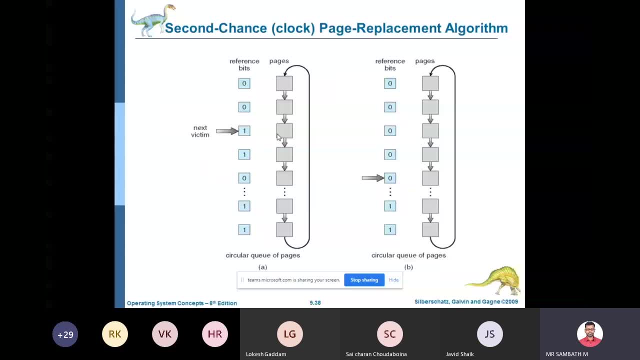 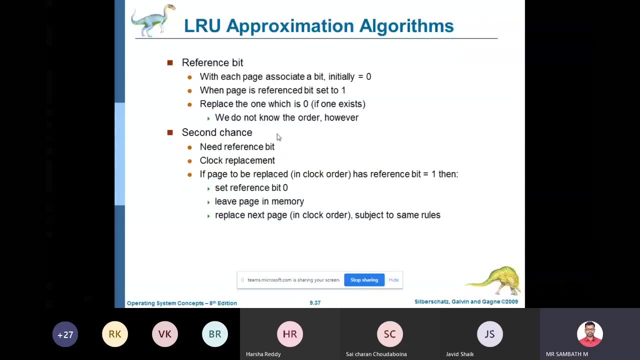 it means that the page is not referred, so i will replace that page- the second chance algorithm- with reference bit. they will attach something called clap. that is a timing at which time the page is referred. so they will check the reference bit whether it is one or zero. 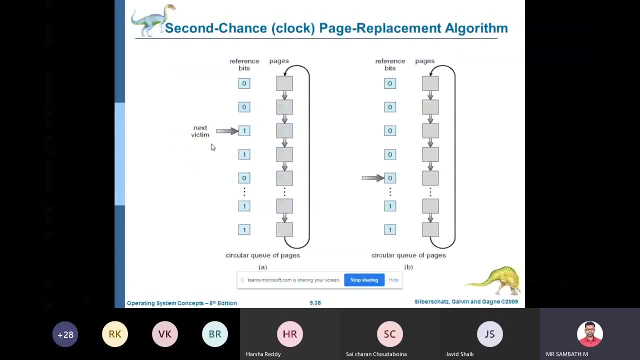 even if it is one, they will check the timing at what time the page is referred. ok, so if the time is previously, that is, long before, then they will remove that page. that is the second chance. so in reference bit they will check only for bit. the second chance: they will check for timing also. 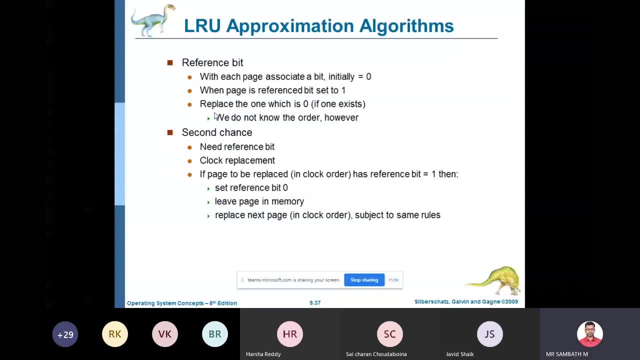 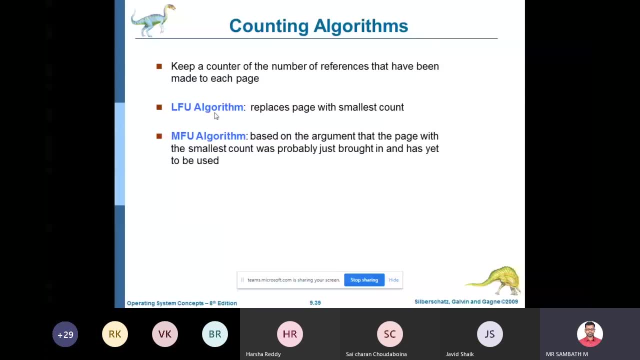 then counting algorithms. in counting algorithms, there are two algorithms available. that is, a least frequently used algorithm, then most frequently used algorithm. so, as the algorithm name indicates, lfu algorithm, replace the page with smallest count. they are going to maintain a counter for each page, keep a counter of the number of references that have been made to each page. 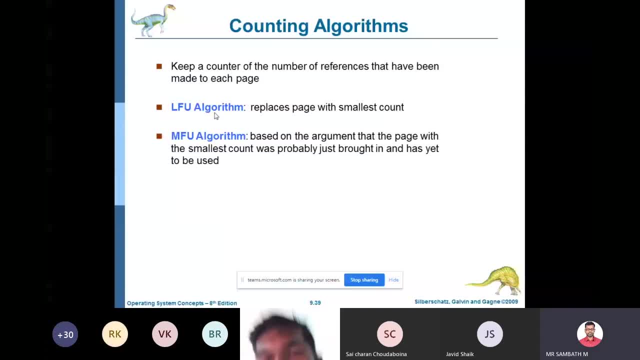 ok, so here which page you will replace, according to lfu, the page which is having smallest count. why? because if the page is having smallest count, it means that the page is referred for less number of times, so it means that there is no use of that page. 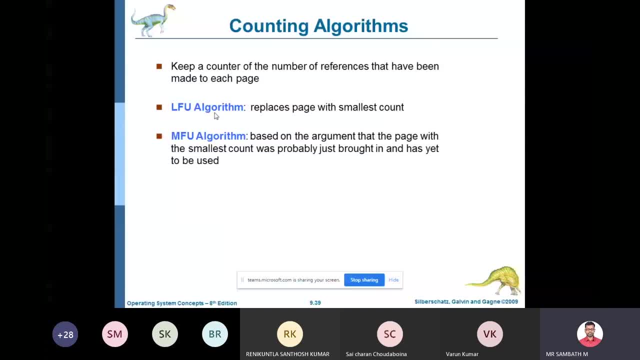 this is not referred oftenly, so remove that page. that is what the lfu algorithm says. but when you go for mfu algorithm- that is the most frequently used algorithm- you will remove the page with higher count. ok, that is the which is having the large count. 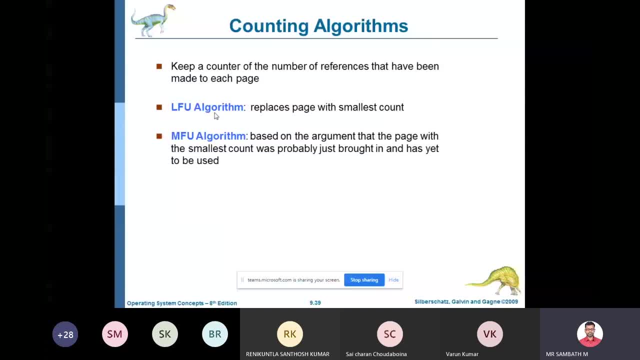 why? because the page is going to be removed if the page is having higher count. why? because they are assuming that if the page is referred for large number of times, they will assume that this page is not going to be used in the future. so that is what the assumption is. 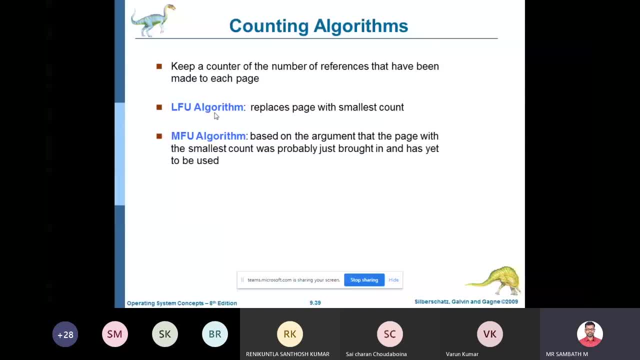 according to this algorithm. so mfu algorithm assumes that if the counter is high, this page is referred enough number of times so it will not be needed in future. so according to this technique, they are removing the page which is having highest number of count. so that is the two algorithm. 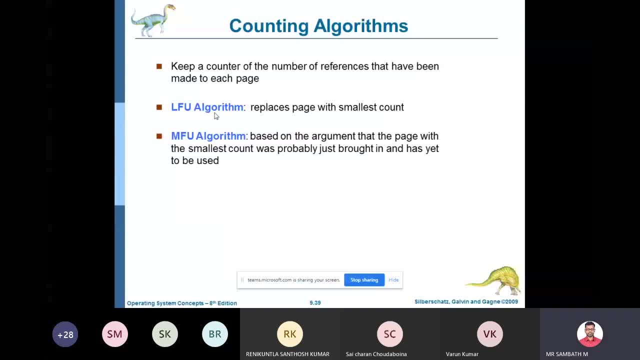 lfu and mfu, but both the algorithms are contradictory. lfu algorithm removes the page with smallest count. why? because it assumes that this page will not be needed, because it is having very less reference. so that is their assumption and this is their assumption. so that is about the algorithms. 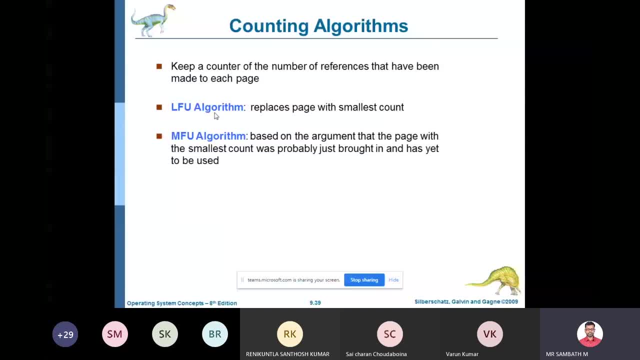 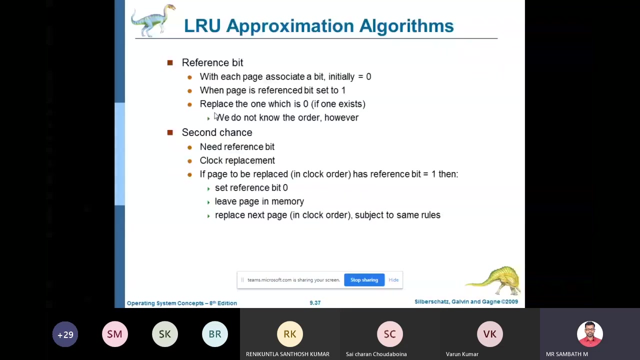 page replacement. so what are the algorithms before? optimal before is first in, first out. optimal is: look at the future reference, next numbers: lru. look back past reference, then lru, approximation reference bit, using reference bit, then counting algorithm least frequently and most frequently, the next we have: 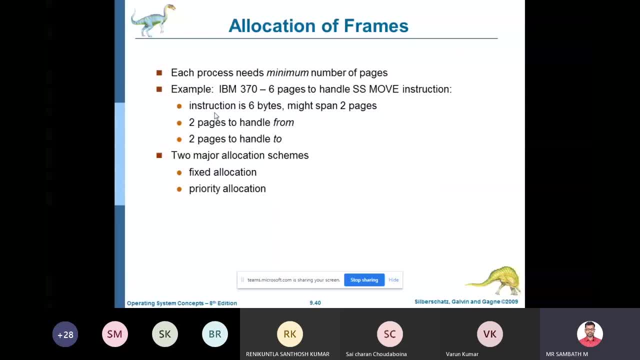 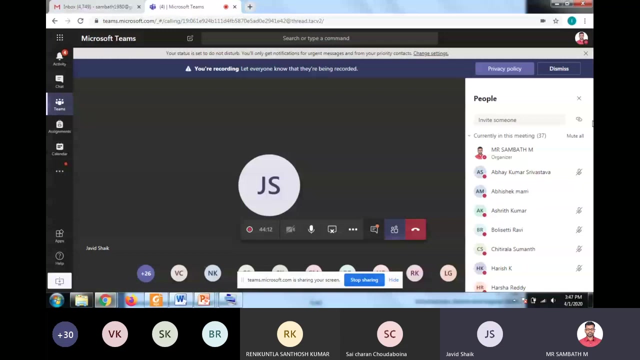 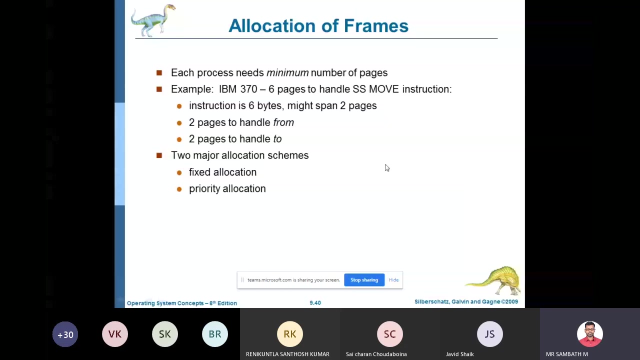 something called allocation of frames. for example, you have a number of processes running how the memory is going to be allotted to the someone is removing from reading. sir, this is fourth or fifth time, sir. hello sir, i will continue. there are basically two major schemes available. one is fixed allocation and priority allocation. 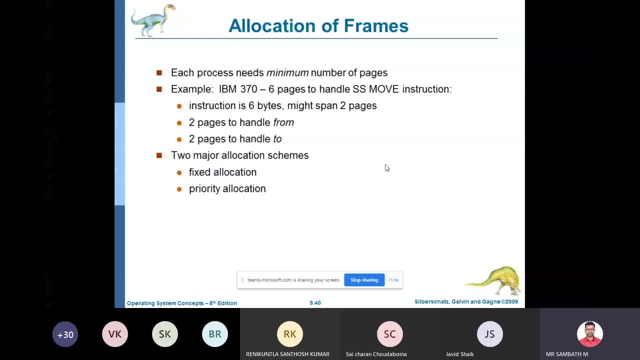 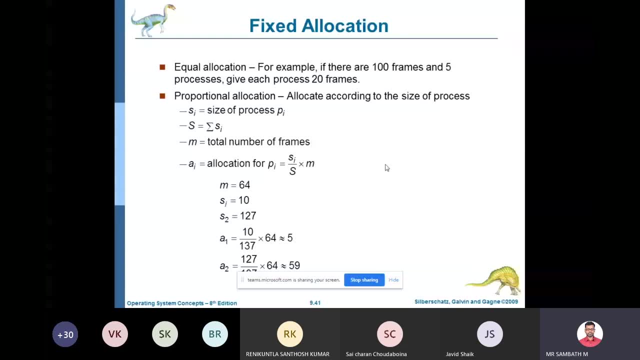 so, according to fixed allocation, how they are going to allocate the memory is: there are two techniques in fixed allocation. one is equal allocation. the second one is proportional allocation. equal allocation is, for example, there are five process available, five process and there are only hundred frames available in the memory. 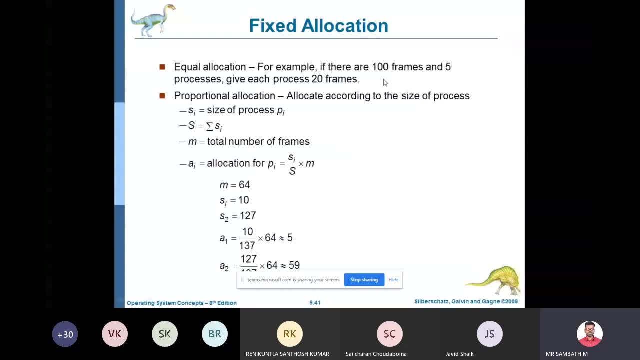 then how you are going to divide it: hundred frames divided by five process, so each process will get twenty frames. ok, so this is how the equal allocation techniques works: just divide by number of process and give it to all the process: twenty frames. twenty frames, so each process will get equal number of memory. 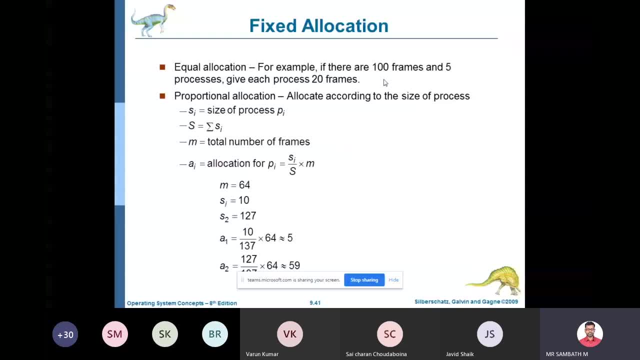 but in proportional allocation. what happens is according to the size of the process it is going to be allocated. ok, now imagine there are sixty four frames available, m equal to sixty four, total number of frames, and there are two. and there are two process available, that is, one and two. 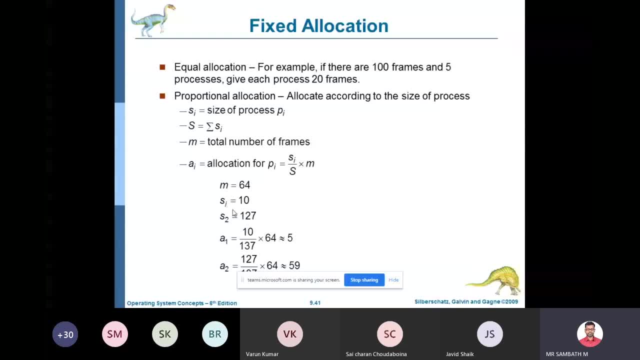 that is, s one is the size of the first process and s two is the size of the second process. so s one is ten and s two is one twenty seven. that is the s one size is ten mb or kb, whatever you keep, and s two is one twenty seven. 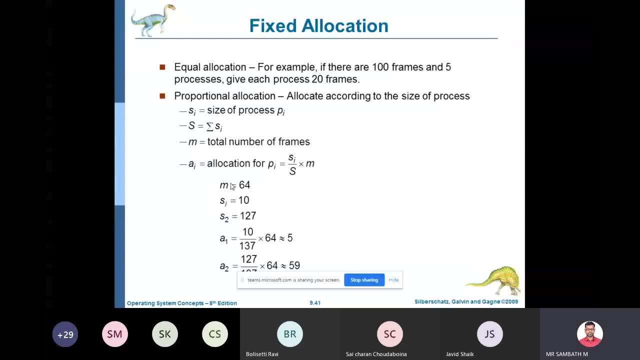 that is one twenty seven kb. imagine, ok now how this sixty four- there are only sixty four frames available- how the sixty four frames are going to be allotted to process p one and p two, that is, s one and s two. s one and s two is the size of the process, p one and p two. 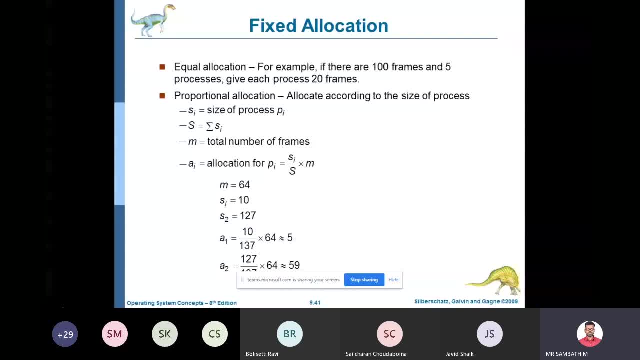 so there is a form law, a one equal to ten. ten is the size of the first process divided by one thirty seven. what is that? one thirty seven, one thirty seven is the total size of both the process. ten plus one twenty seven. ten plus one twenty seven, that is one thirty seven. 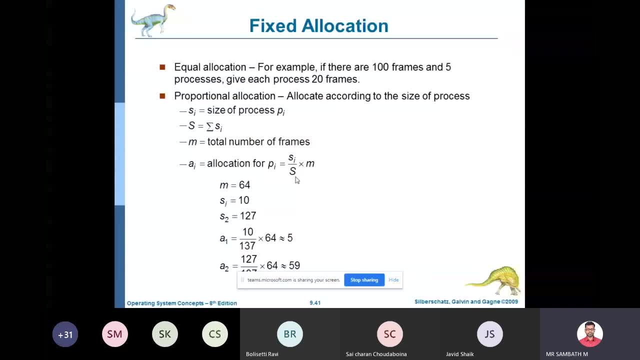 into sixty four. sixty four is the number of frames available. so if you do this calculation you will get five. so five frames are allocated to process p one which is having size ten. ok, the next process. next process is eight a two equal to one twenty seven divided by one thirty seven into sixty four. 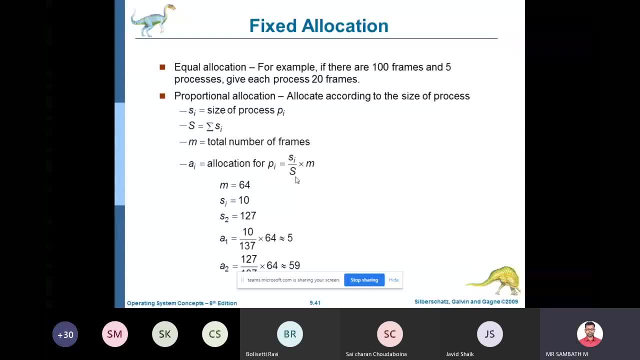 you will get fifty nine. so one twenty seven is the size of the second process divided by the total size of both the process. one twenty seven. that is one thirty seven into sixty four, you will get fifty nine. so fifty nine frames are allocated to second process, which is having size one twenty seven. 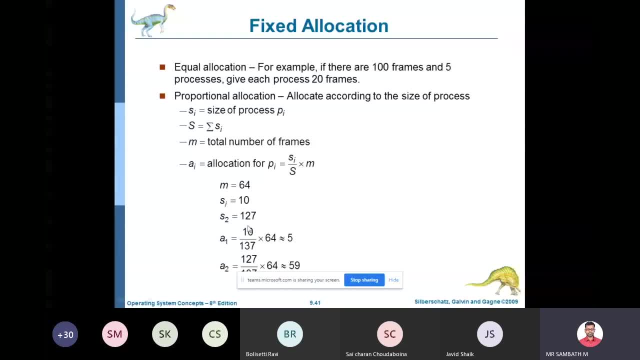 and five frames are allotted to first process which is having size ten, so fifty nine plus four, sixty four. so sixty four is divided like this. this is called proportional allocation, according to the size they are allocated. so these both the techniques coming under fixed allocation. the next one is priority allocation. 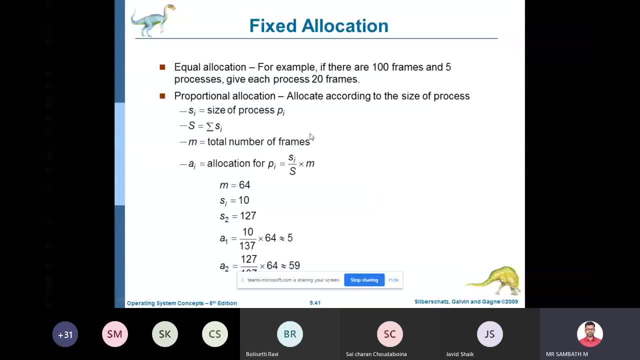 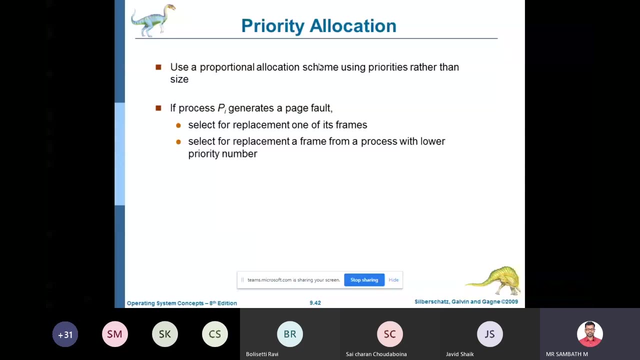 in priority allocation. here they are using the size to allocate, but in priority allocation they are going to use the priority. for example, p one is having highest priority one and p two is having lowest priority, then p one will be given with, for example, it may be fifty nine frames. 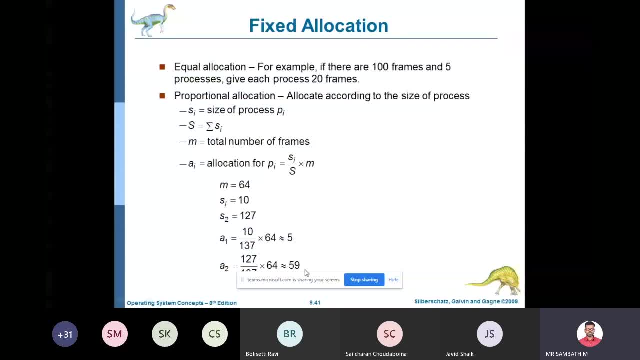 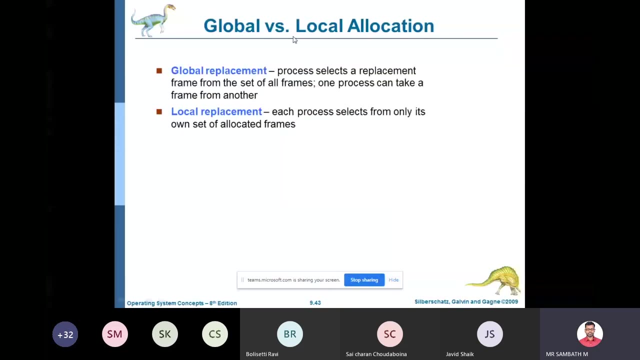 and p two will be given with five frames. so according to the priority they will allocate the memory here, according to the size they are allocating the memory. so that is why it is called priority allocation. the next one: we have global replacement and local replacement. global replacement is like: 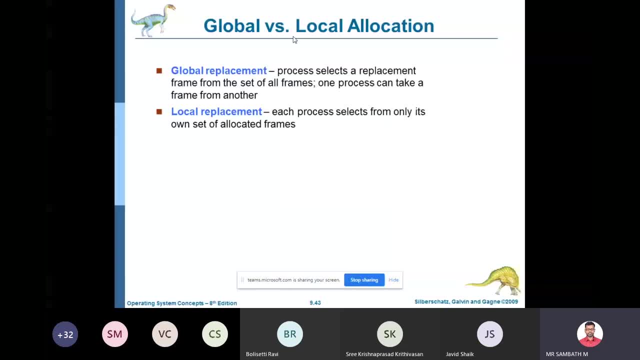 the process. select a replacement frame from the set of. there are, for example, there are five frames, sorry, five process running. there are the process. want to do the page replacement? then what it will do now: it will replace the page which is available in any of the process. 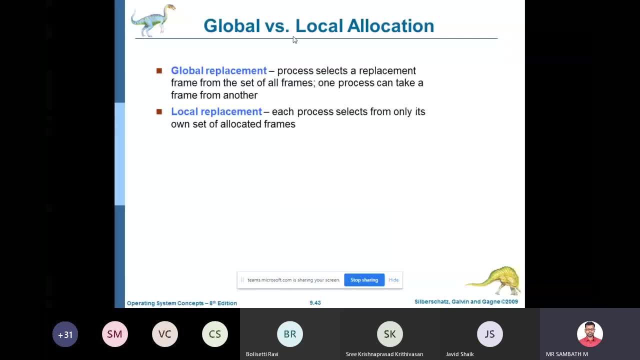 that is called global pay replacement, but local replacement. the process will replace the page only within the pages which is allotted to that process alone. that is the local replacement. the process selects from only its own set of allocated frames. the process will replace the page within its own frames. 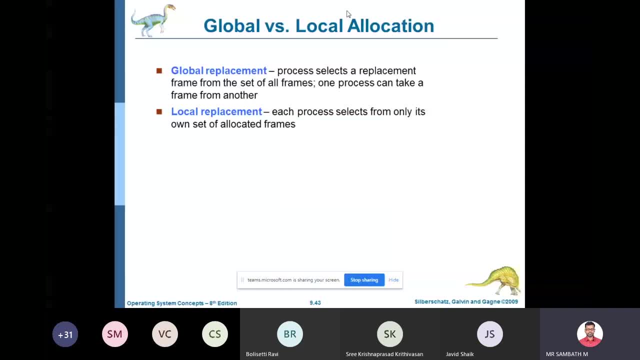 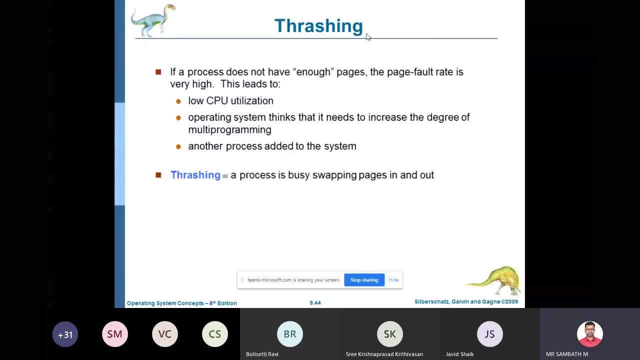 it cannot go for other process pages, so that is called local replacement. the next concept we have called thrashing. thrashing is nothing, but you can say busy in paging. so what do you mean by paging? paging is nothing but mapping, mapping the data from the hard disk. 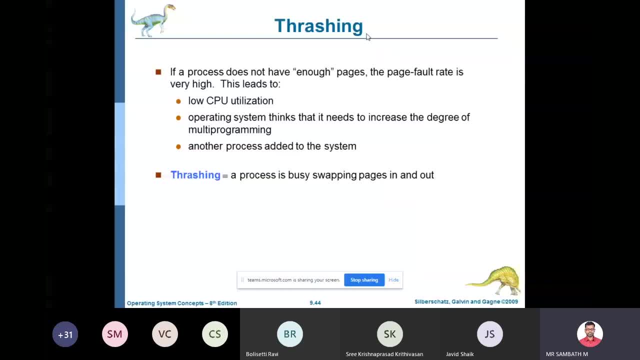 into the main memory. so whenever there is a page fault, the process will go to the operating system, will go to the hard disk and it will bring in the page into the main memory. now, when the page fault is more, what will happen? it means that the pages are not available in the memory. 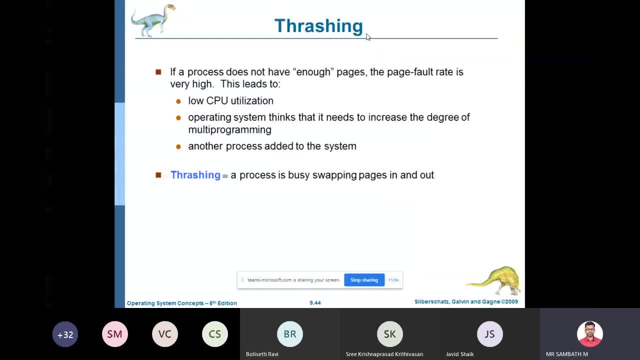 so the operating system will keep on go to the hard disk and it will keep on bring the page whenever there is more page fault. more page fault means the more number of pages are not available. so it will again and again it will go to the hard disk. 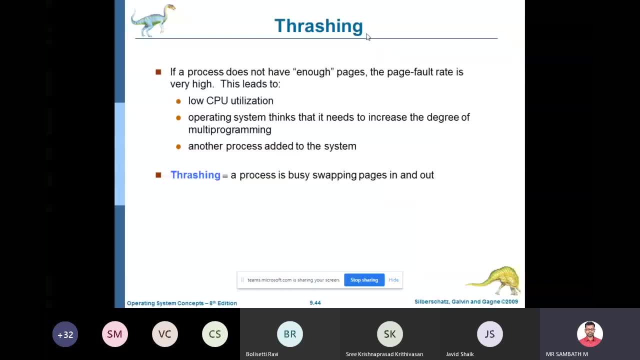 again and again. it will bring the page inside into the memory. so, because of this, what will happen is there will be a high level paging activity will happen. so thrashing in simple terms, it is called as high level paging activity. instead of executing the program, the cpu, what it will do now, 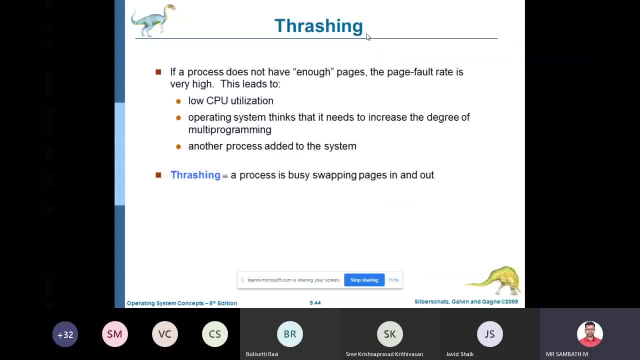 the cpu will keep on, go to the hard disk and it will bring the page. so this, only this paging will takes place instead of executing the program. the paging will be more. so this activity is called thrashing. so thrashing a process is busy, swapping the pages in and out. 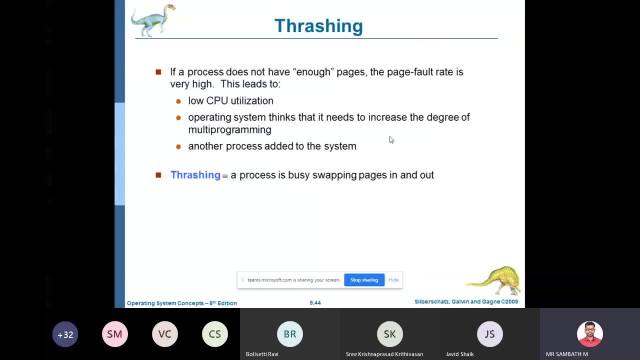 so the process will keep on swap the pages in and out instead of executing the process. so this concept is called thrashing. so whenever there is a more page fault the process, the os will go to the hard disk and it will keep on doing the pages inside. 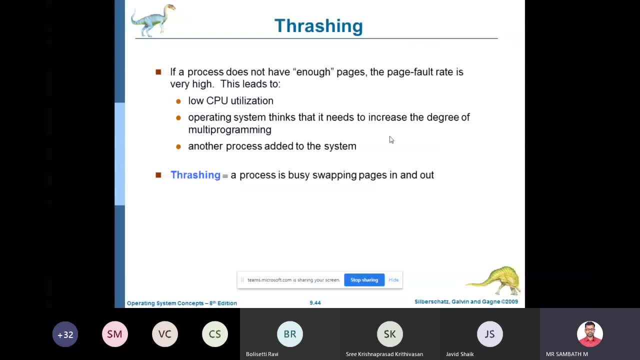 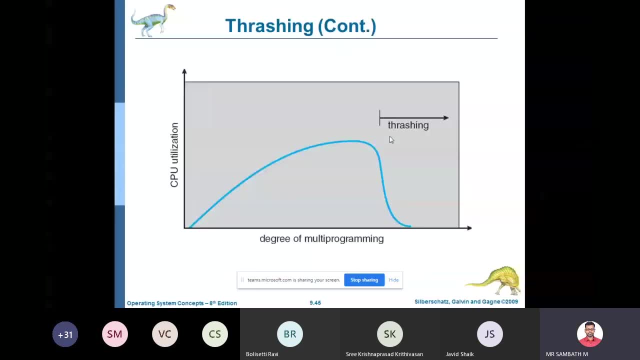 so this is the high level paging. this is one important 2 mark question. it may come in 2 mark or 6 mark also. what is thrashing? so that is thrashing in simple terms, called high level paging activity. so with this, this chapter is getting over. 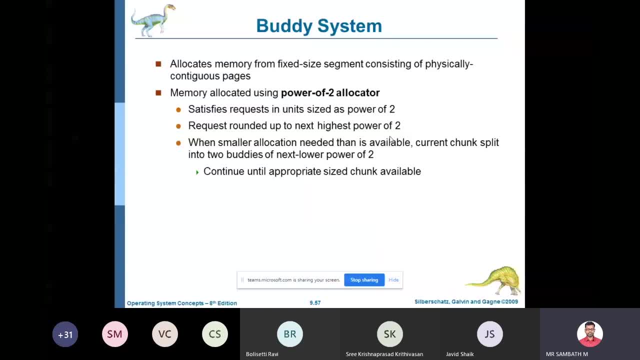 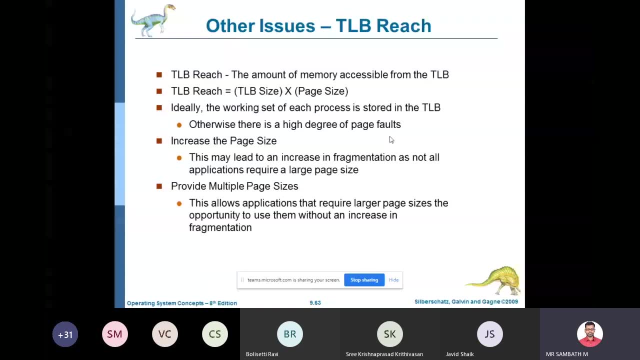 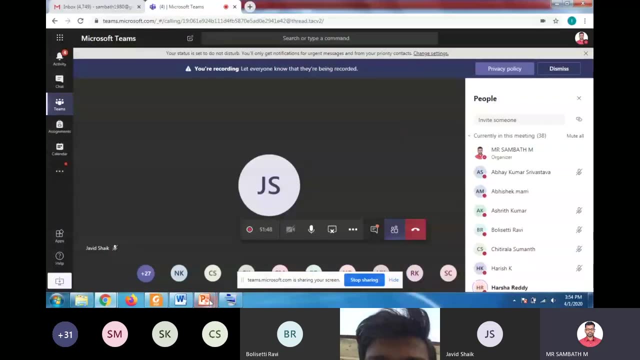 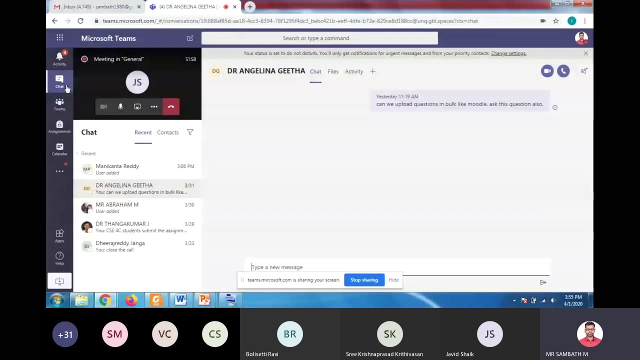 so we will see. we will see the next topics in the next class. thank you, sir. you have a chat box. yes, one see the chat box. chat box, yes, sir. why see sir? sir, one see one. see the chat box. who is writing it? yes, sir, welcome, welcome. 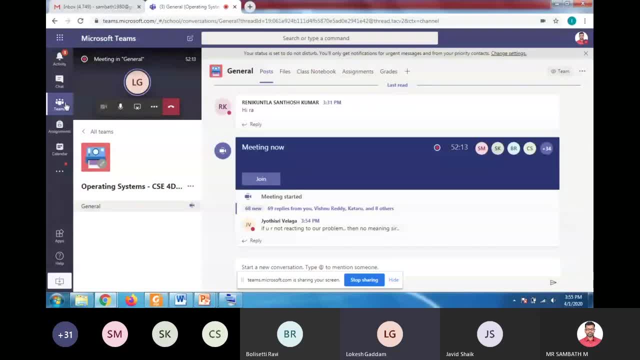 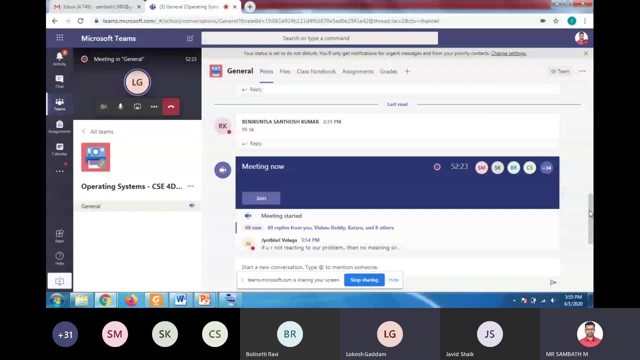 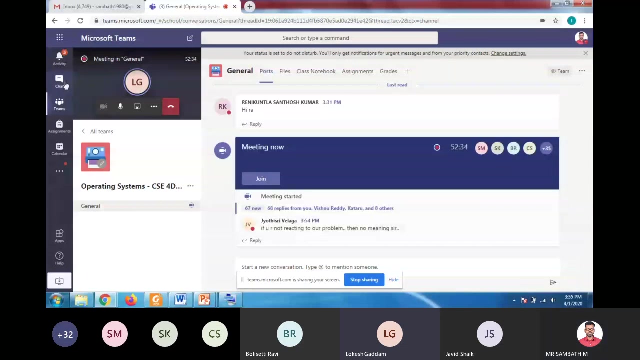 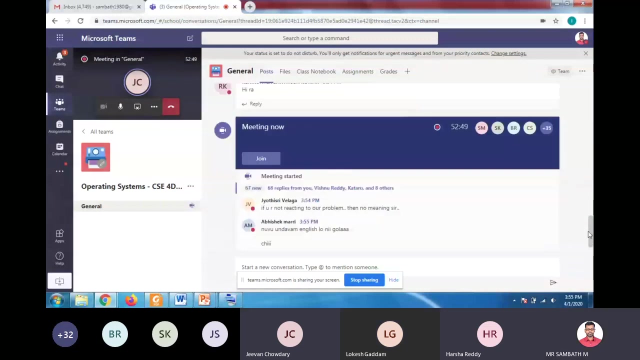 welcome, welcome, welcome, hi, welcome, welcome, welcome, welcome. Jyoti Shree has returned, Sir, Sir, everyone, someone is Santosh Santosh sir, Jyoti Shree. Yes, sir, That one is Jyoti Shree, Santosh everyone, Everyone Santosh, sir. I don't know how to avoid this problem. 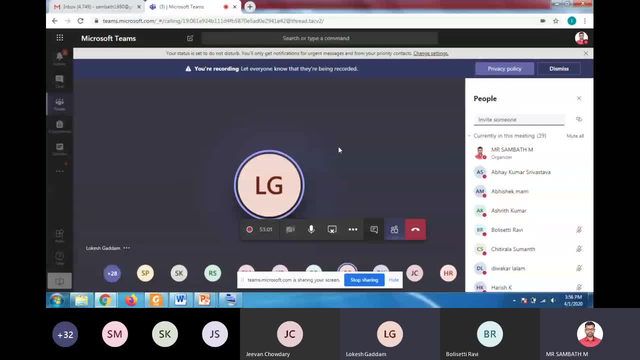 Santosh. sir, See you, people have to behave properly. I don't know what is the solution to this problem. Santosh, behave properly. I already told you. Hey, Chiran, Leave the meeting. He is winning Chiran, sir, Sir, we are entering our records, Sir. what, sir? You have to complete your records when you are coming. 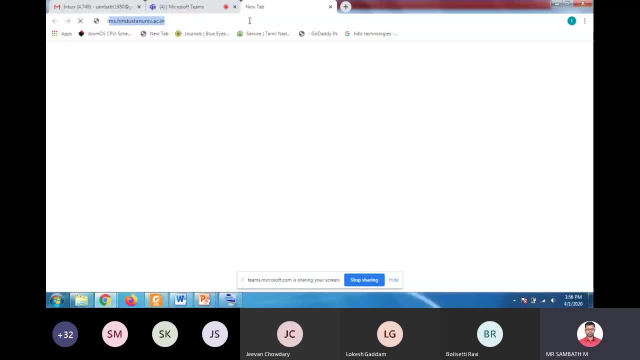 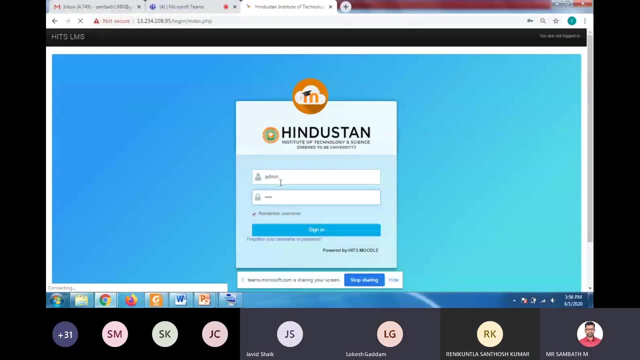 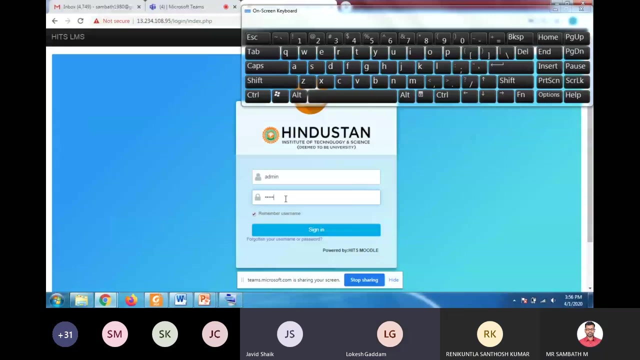 OS lab records. Sir, sir Jeevam, please don't remove me. What, Sir? We are in the room? Tell me We are not recording, Sir, Why I took it. sir, You said hot for 10 days. We don't know it will extend for another 10 days. 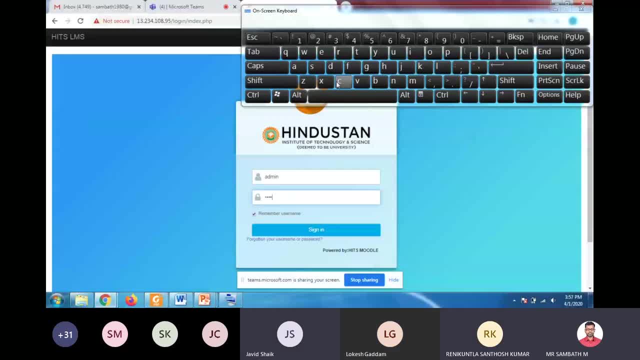 Where is your records now? In Chennai, sir? Chennai, Sir, it will extend, We thought till 31st only, So we kept there only. Ok, Whoever is having the record, You finish it Ok In the In the moodle lms. I have uploaded the programs also. Ok, sir. 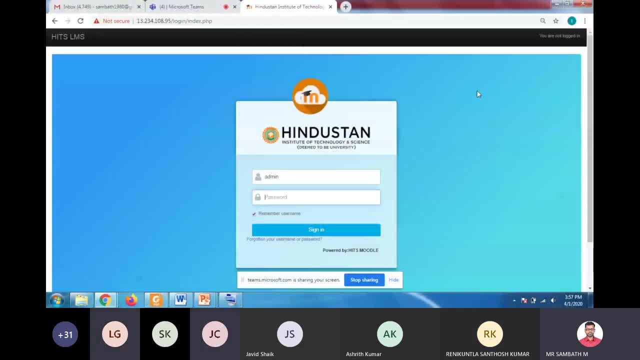 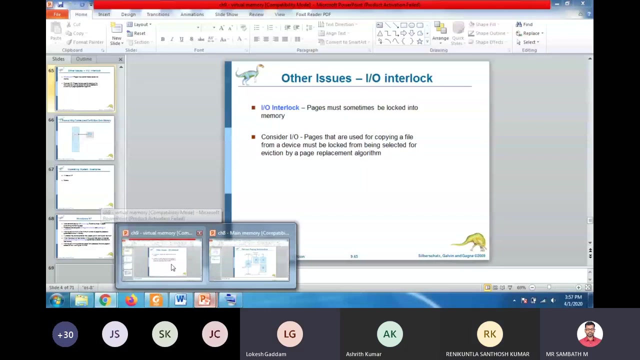 You can write till: What is that Arsha? what is the last program, Sir? page replacement algorithm. No, page replacement algorithm. You no need to write Arsha. is it working or not, Sir? you send sir Order Order. No, you go to One second. Arsha, did you return? 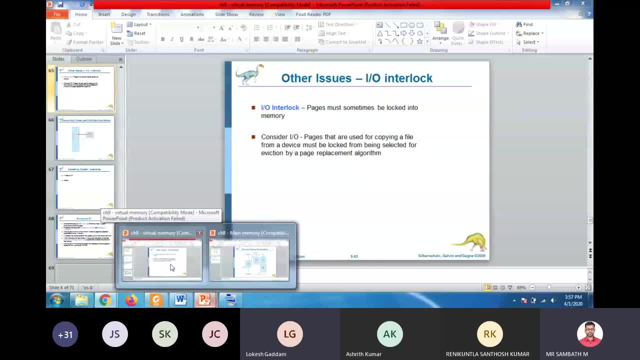 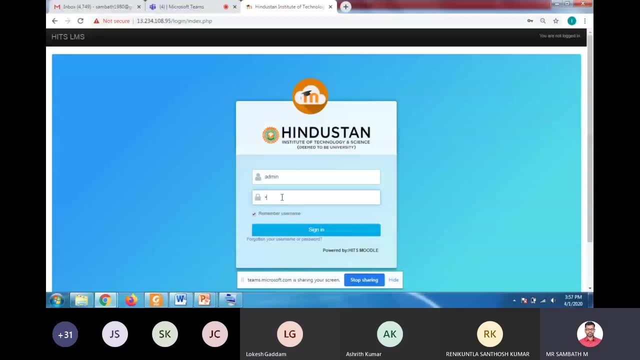 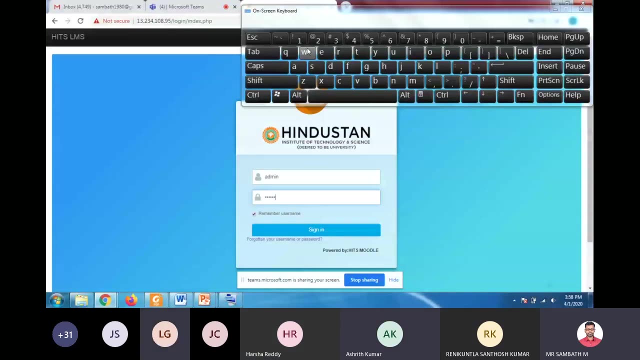 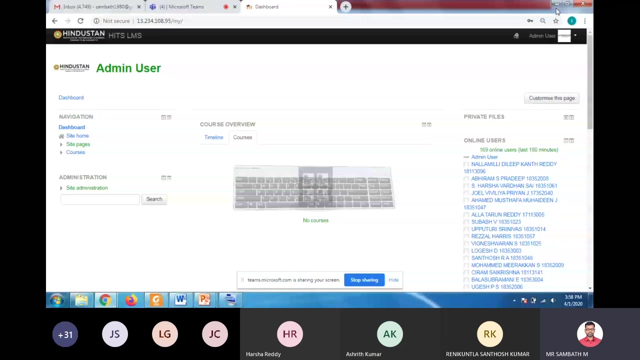 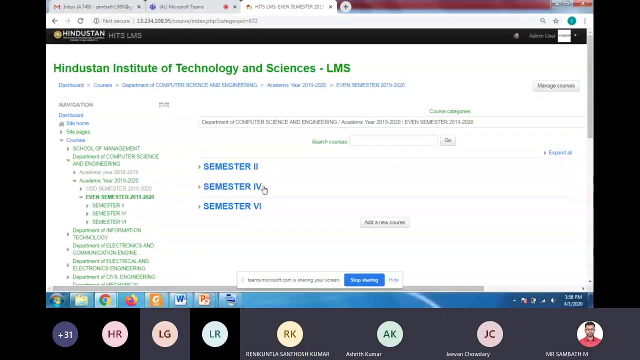 Sir, Sir, Almost, sir, Almost sir. What is the last program, Sir? create process and threads. Yeah, create process and Threads, Threads. I will show you now. Wait, wait, Sir. Department of computer science, Jeevan. please don't remove me. Ok, Sir, Tell me the people Who are all removing, like this: 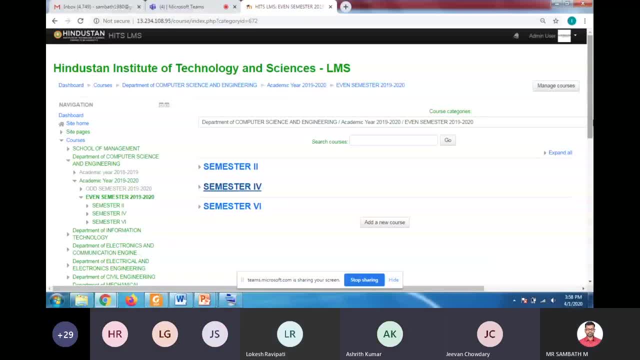 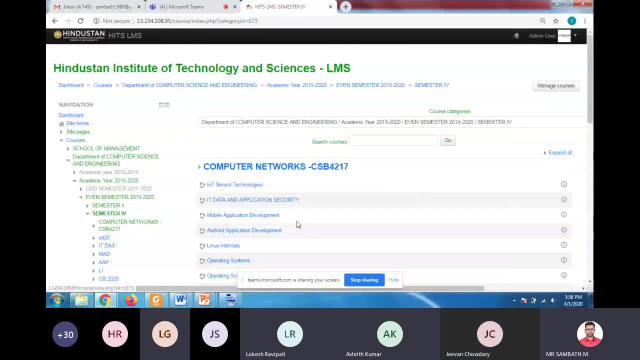 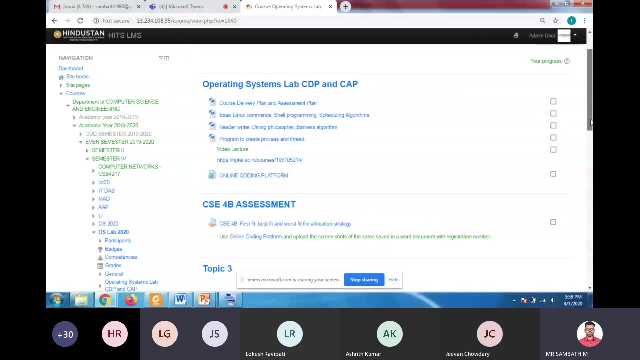 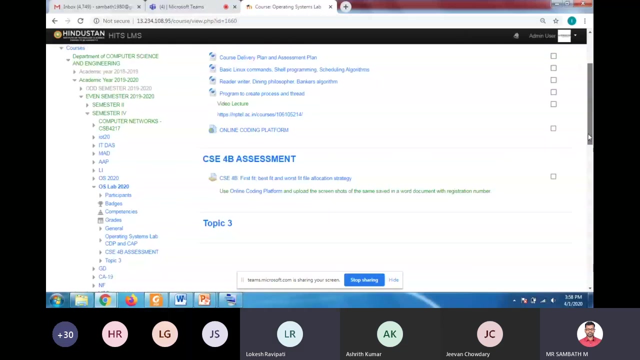 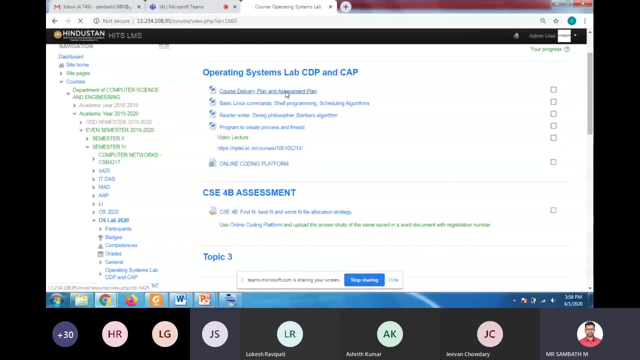 I will remove them. Wait, can they, Sir, Next time? Next time I will remove Santosh Jeevan, sir Javi, sir, Sir Srinivas Mumbai. also sir, Sir, Sir 4 나. Sir Арusa Arsa, sir Arsa, Arsa, Arsa, Arsa. 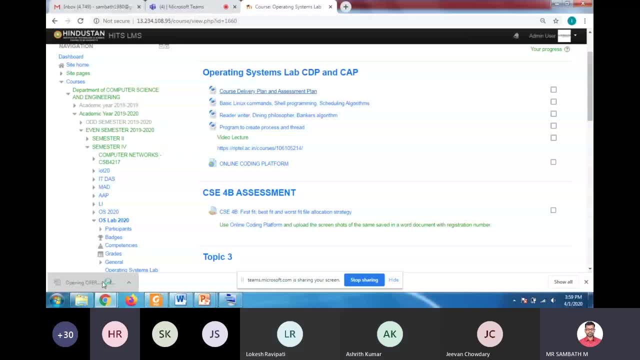 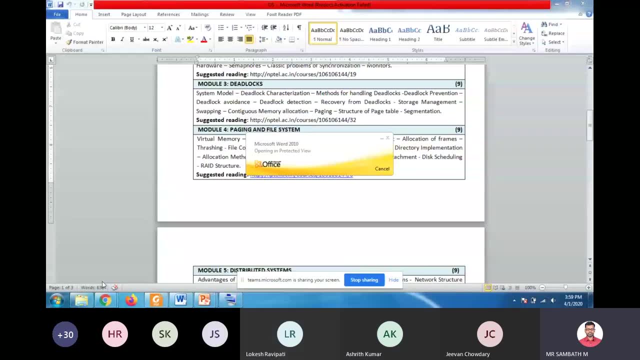 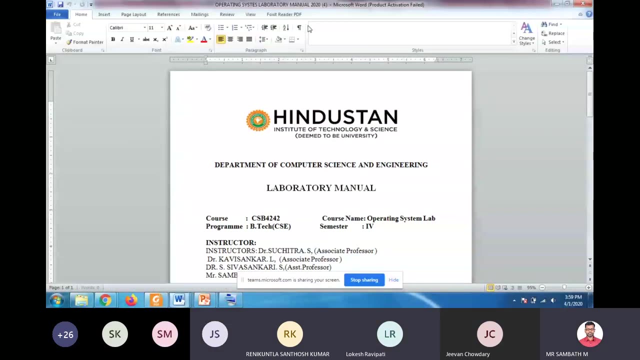 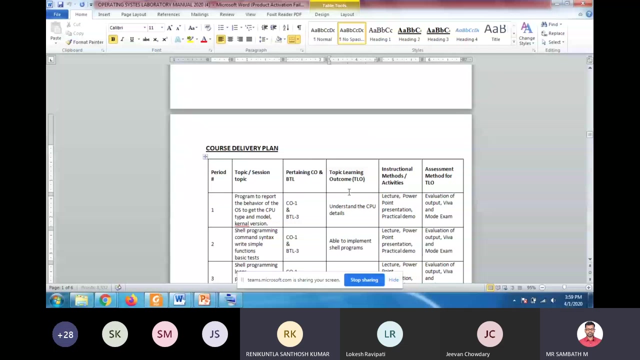 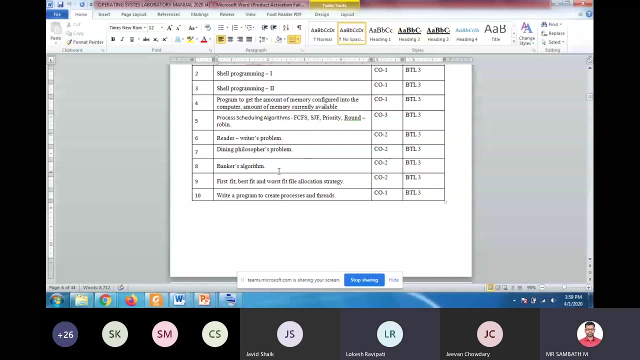 Arsa, Arsa, Sir, Arse, Arse, Arse, You have already completed TIL Bankers Algorithm, right? Yes, sir, Okay, First fit, best fit, worst fit. you have to do then create process and threads. So this is the last program. 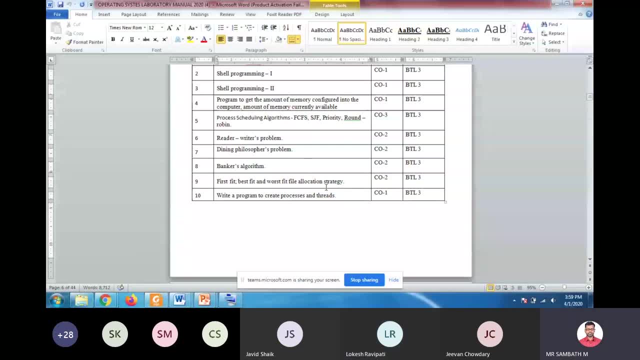 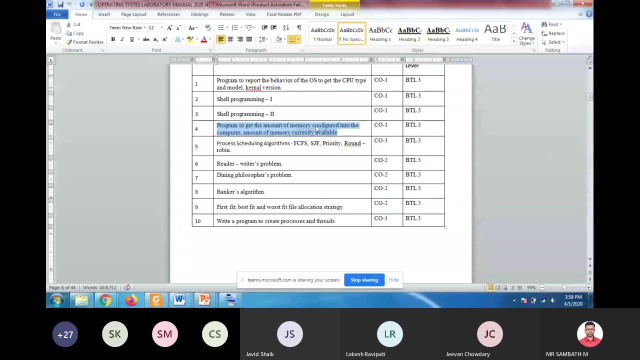 And after this I think we left this program. That is the fourth program we will do: Program to get the amount of memory configured into the computer and the amount of memory are currently available. So this also you should write at the last. 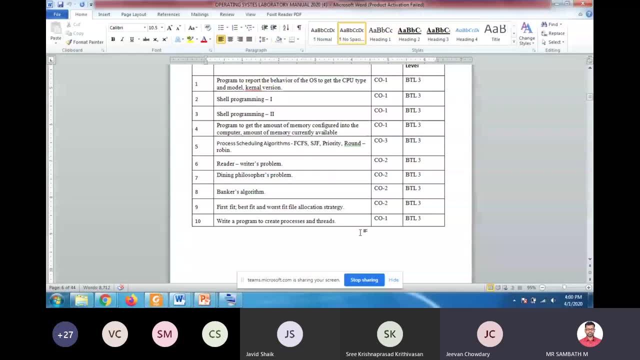 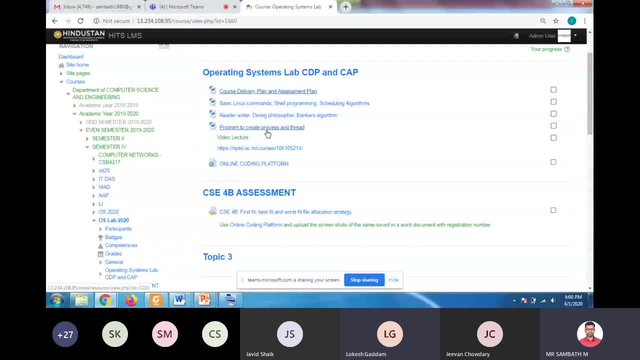 Okay, sir, Okay sir, Okay, sir, One, and then you will complete this month's program. Okay, sir, Program also will have been given here. Okay, Okay, sir, All the programs will be given here, okay. 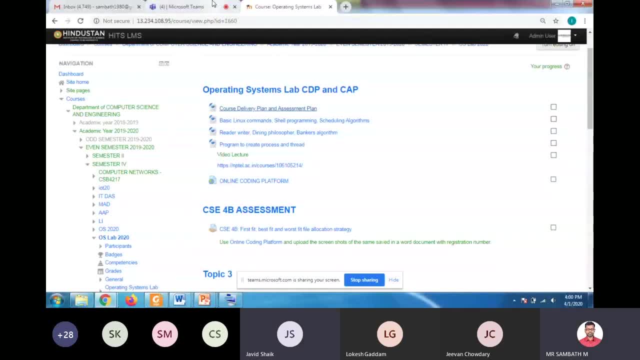 So complete the record before coming here. Okay sir, Okay sir, Then we will meet. Try to finish this environments. All this will take time, or sir? No, I told that one. Enjoy to everyone, sir. See you later. 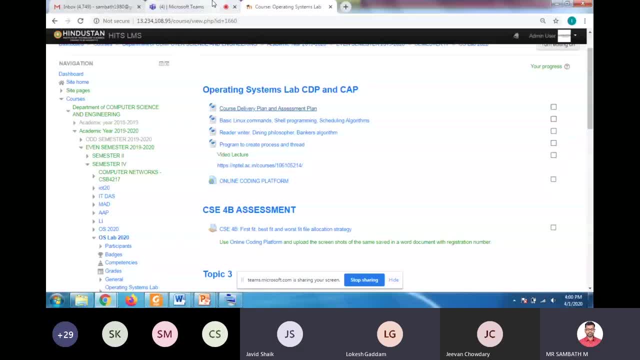 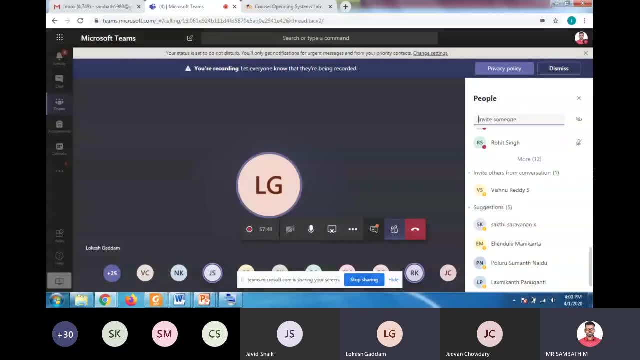 Bye sir, Bye sir, Bye, bye, Bye everyone. Bye, Bye, bye sir. Thank you, sir. Thank you, madam Sindhu sir. Thank you, Take care, Thank you. addicted actually, Sir. please look at the chat, sir. 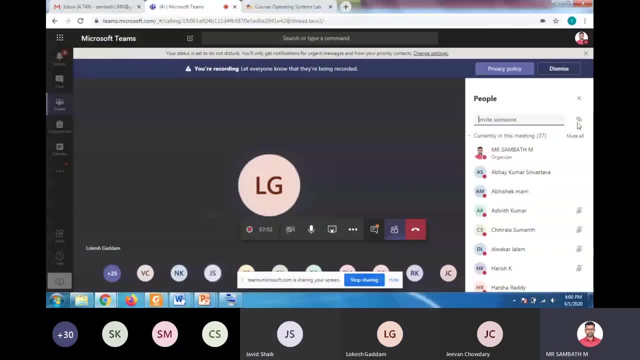 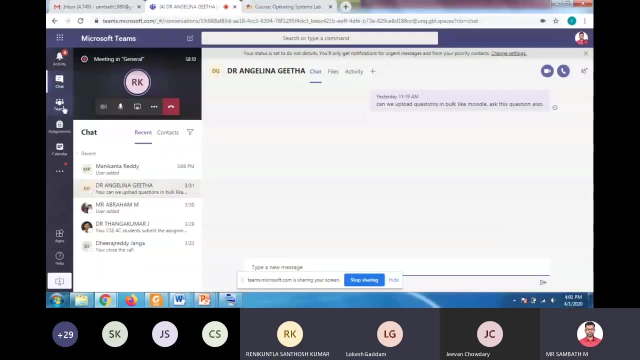 What? Look at the chat, sir. Sir, look at the chat, sir. What is there in the chat? We are not able to follow you, sir, today. Bye, Hello, Sir. if you want to come again, you can choose. 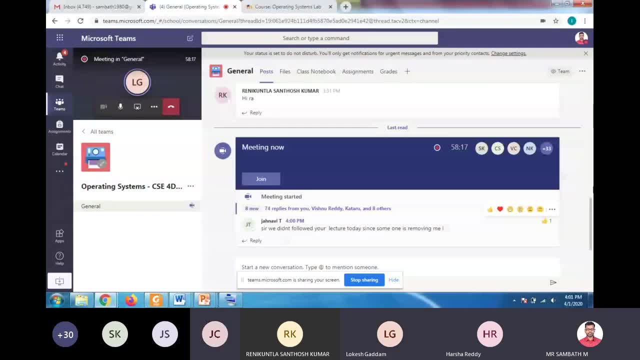 Guys, you can again visit this and you can listen. Okay, sir. thank you, Santosh, Tell me What. What are you writing? I am writing something. I am writing something. Ok, shall we close? No, sir, What are you writing? Kothi Na Koduku Sarva. 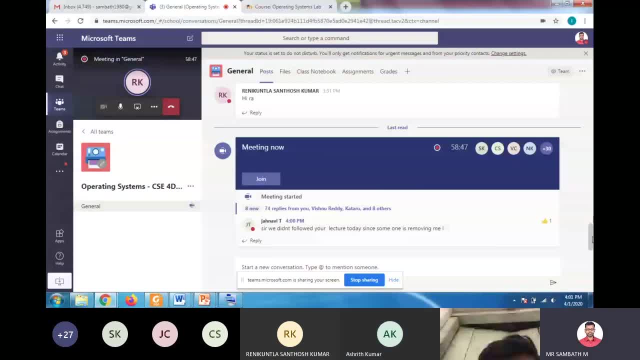 Kothi Na Koduku Sarva. Yes, sir, Next class I am going to remove the people who are doing this kind of Santosh, Santosh. I am removing Hey, hey, Sir, what are you doing? Ok, then Next class we will have another class. Ok, submit your assignments. 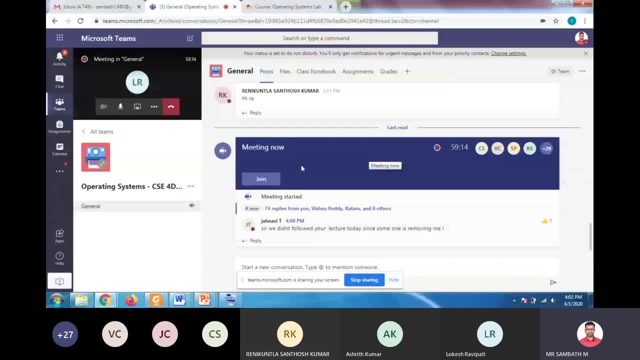 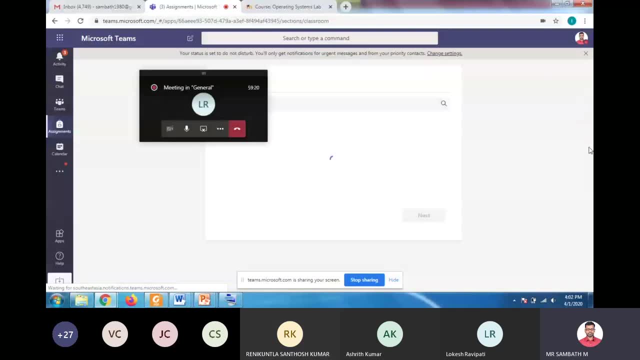 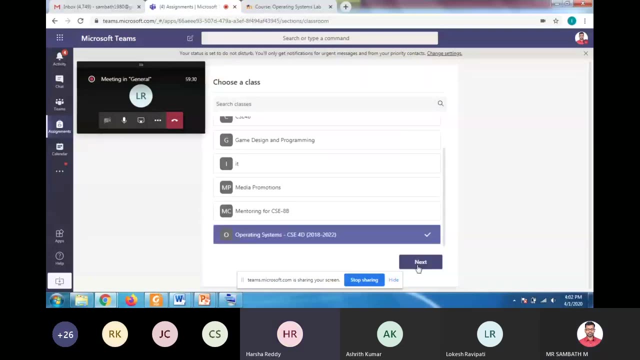 as I said. See, I want to see your assignments here. Tell me. tell me, Sir. in files you can see those who submitted. no need to submit there In files. those who submitted it will show there. Ok wait, let me check. Ok wait, let me check, Sir Santosh. 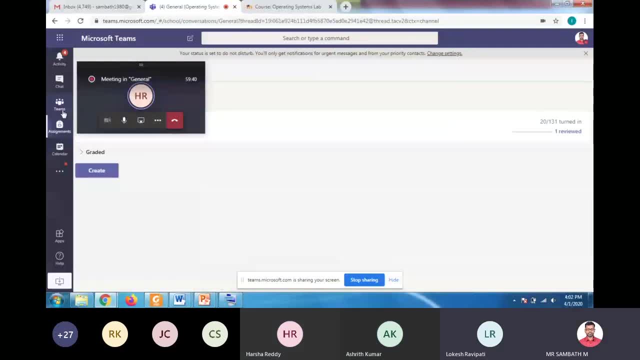 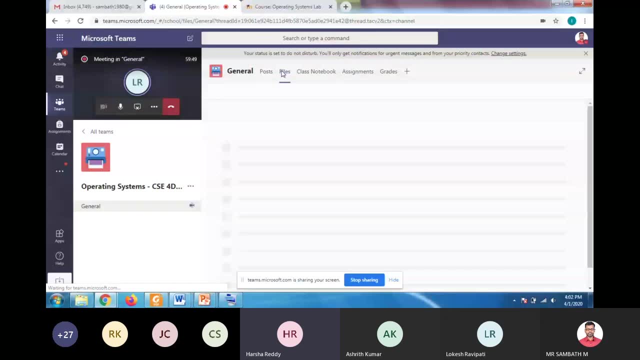 Santosh not submitted till now. Santosh not submitted till now. Yes, sir, files in that those who submitted it will show there. Ok, ok, Ok, then let me What is the first thing happening, sir? Everyone is submitted by Asha Reddy. Yes sir, Yes sir, No sir, no sir. 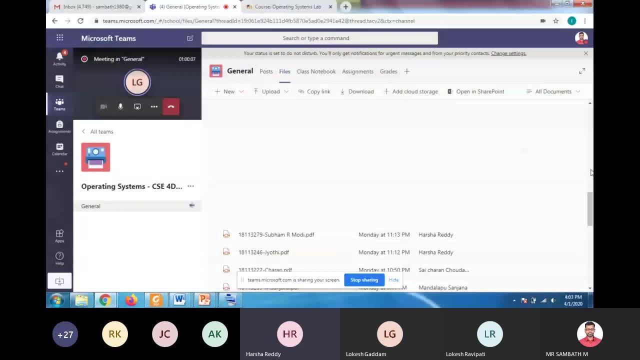 I just modified their name, sir, because if you check, if you go there, means for verification purpose, it is very clean, Asha, Telugu, don't trouble. Ok, wait, sir, wait. Ok, then I will check. Ok, then I will check. Ok, all of you taken the quiz also, no, 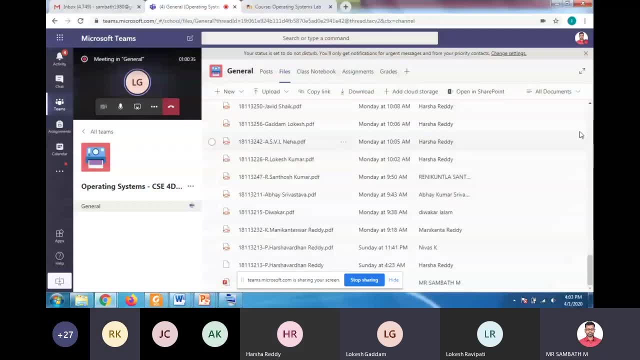 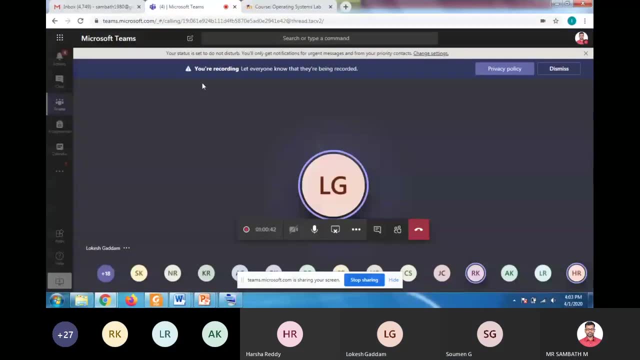 Yes, sir, Sir, Ok, done, ok, Sir, except me. everyone has taken sir. Me also did not take, sir. I will take now. Who is this? Santosh Renekun, Santosh, Santosh Renekun, sir. Santosh Renekun Santosh, didn't take quiz, sir. 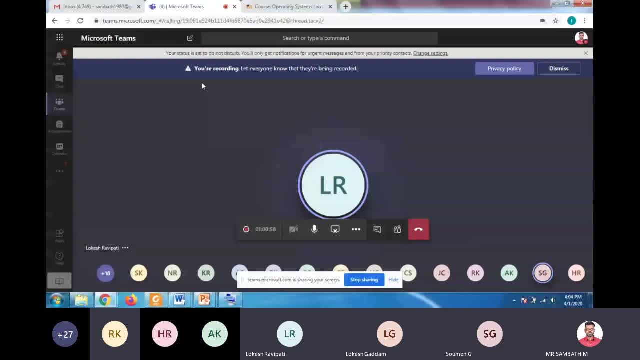 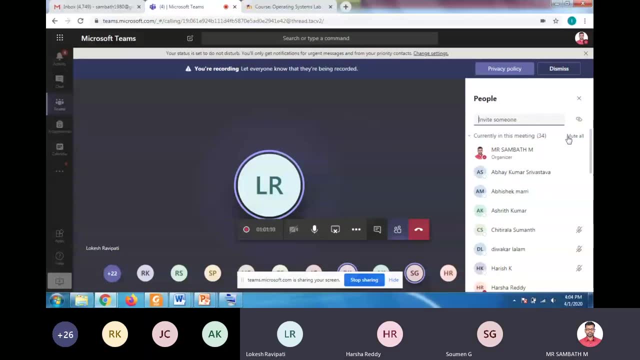 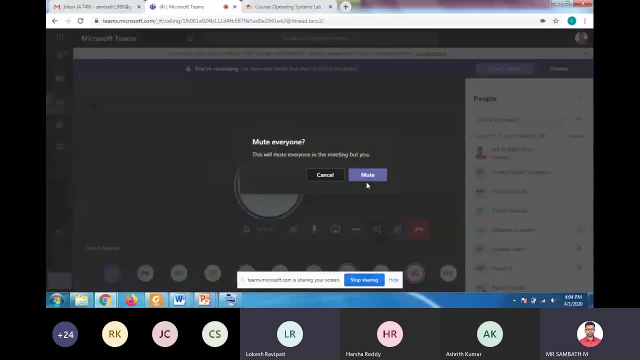 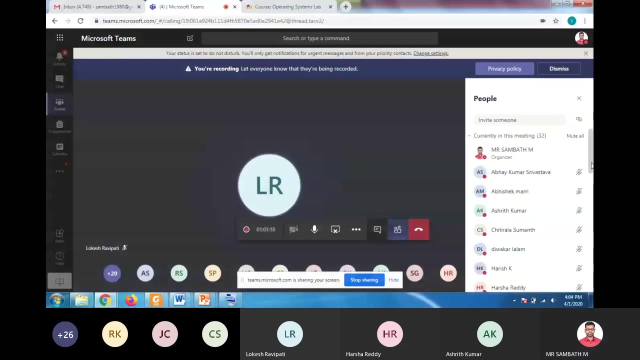 Santosh didn't take quiz. sir, I don't even have here Elements account, sir. I am writing CA in assignment, sir. I am writing CA in assignment, sir. I am writing CA in assignment. sir, Sauman, you alone unmute and talk. Sauman, unmute, Sauman, use mute. 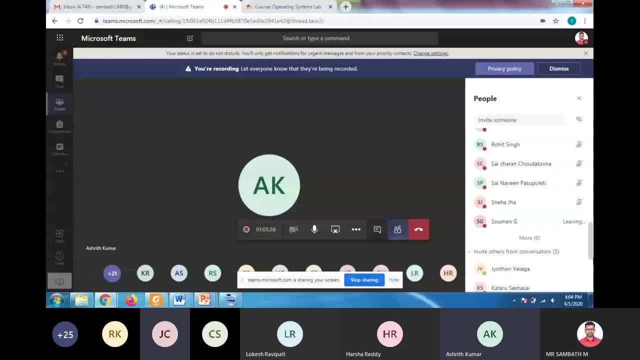 Turn off and talk. Sauman, Sauman town, ADUR LUNCH, ADUR LUNCH known. Had your lunch known You? yes, sir, idi.